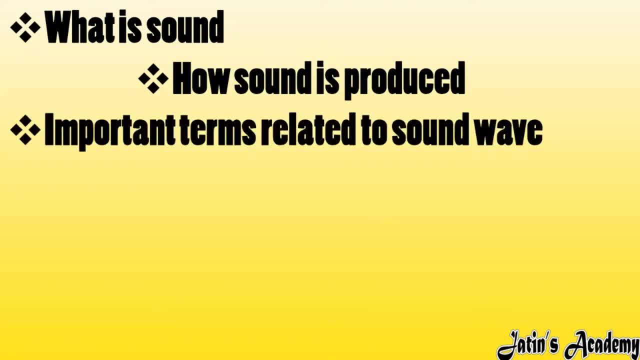 we are going to study about important terms related to sound wave, Then we are having characteristics of sound. In characteristics of sound, we are firstly going to study about pitch, Then we are having loudness, Then we will study about timbre. So very first, 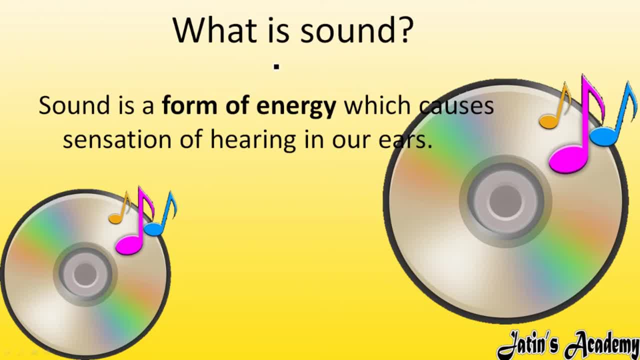 topic we are having what is sound. So first of all, we should know what is sound. So what is sound? As we have read, heat energy, light energy, in the same form, sound is also a form of energy. It means it is a form of energy due to which we feel some sensations. 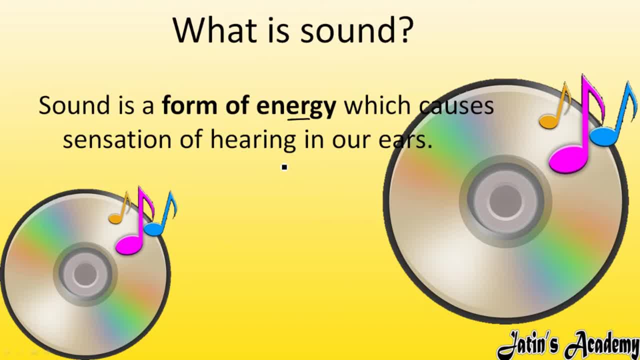 in the ears, That is, some sensation went in our ear and those sensations went in our ears and we thought that, yes, something went in our ear and we heard something. That is what we call sound. So sound is nothing. It is a form of energy which causes sensation. 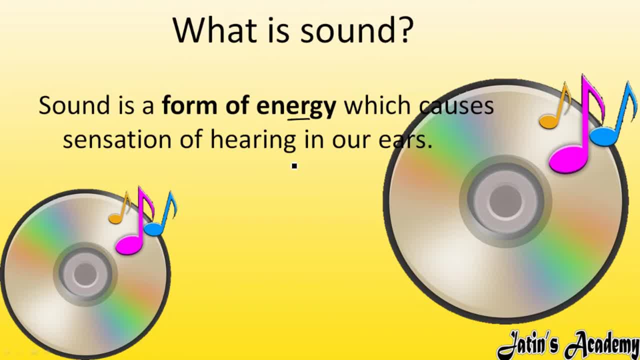 of hearing into our ears. That is known as sound. Okay, So now my question is that: how sound is produced? Actually, how is sound produced? So, how is sound produced? Sound is produced by the vibrations of the object. If I have any object and I strike the object, 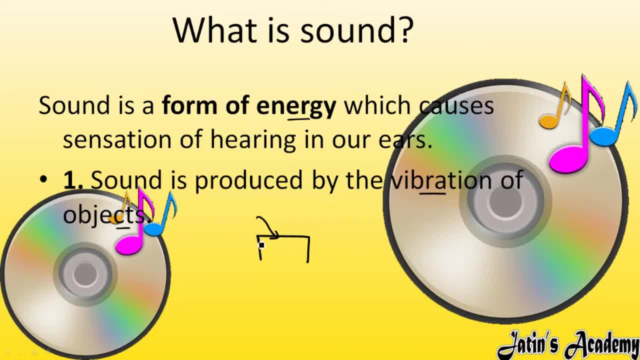 by any object. Okay, What I have done with any object, I have done with any object. So, if the object vibrates, What mean by vibration? That the particles of the object moves to and fro. Now, what is a to and fro? To and fro mean that if any option is turned to, 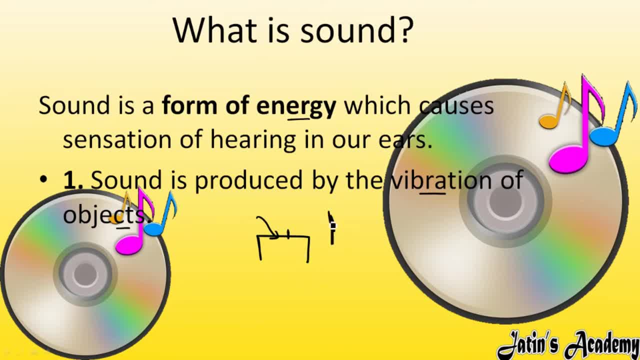 give or move like that. So we call that vibrations To and fro motion. If any particles of the substance will produce this motion, Then we will call that that object is vibrating. So if any object is vibrating, so any changes will occur. there are two changes. The ones: 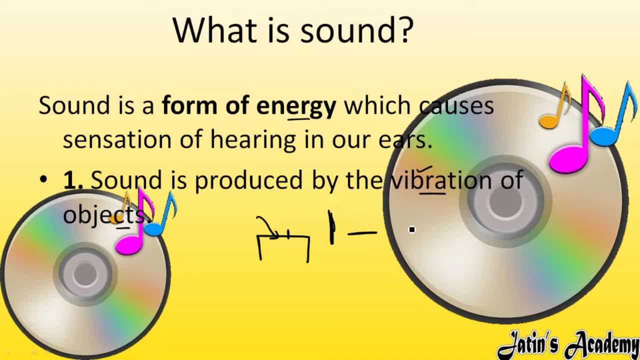 which work is expression? what anything is possible? Next, Is there any change or change? If any, So what will be produced by vibration? Sound will be produced by vibration. So our question is clear that how sound is produced. Sound is produced by the vibrations in any object. 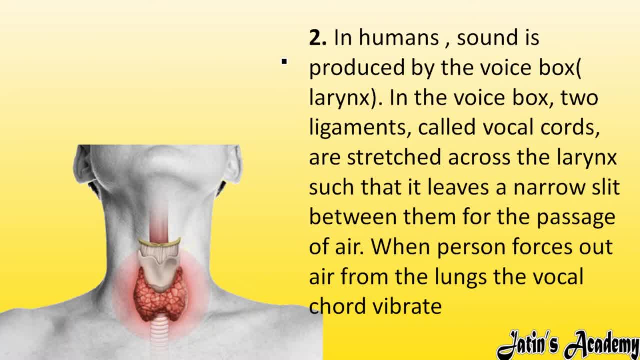 So my next question is that how in humans sound is produced. So how sound is produced in humans. So actually, what happens in humans is that one is under the throat, here is a voice box. We also call voice box as larynx. 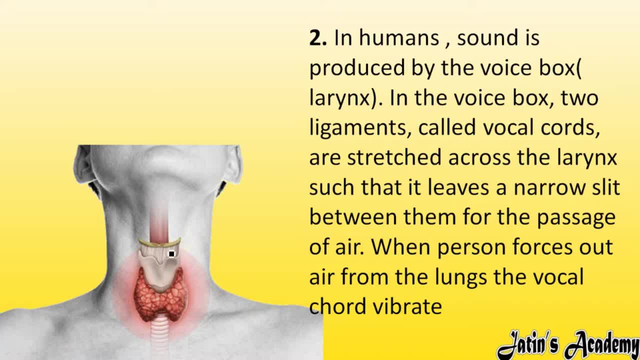 So what happens in voice box? There are two ligaments in voice box. There are two ligaments in this voice box. We call those two ligaments vocal cords. Do you understand? There are two ligaments in voice box And those ligaments are called vocal cords. 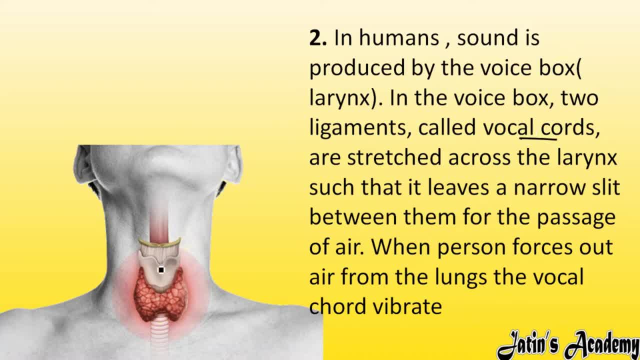 And vocal cords are stretched across the larynx. This is our whole larynx. The portion below the throat is called larynx And the vocal cords are inside the larynx. And what happens in that? There is a narrow slit inside the vocal cords. 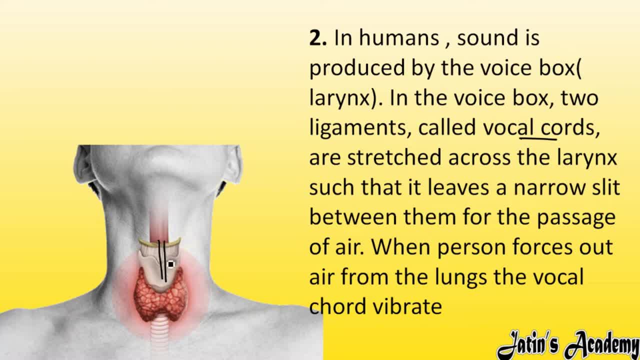 Let's say there is a narrow slit. What happens in that narrow slit? Whenever the air passes through the narrow slit, whenever we try to speak, what happens to our lungs? That air is pushed And that air comes to work. That air comes to work in this narrow slit. 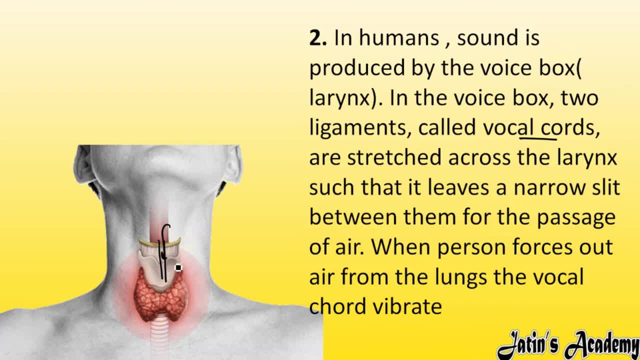 When the air passes through this narrow slit, then our vocal cords start vibrating. when it passes through the air, Because the air will create pressure Means. if it creates pressure, then what will it do? Vocal cords will vibrate, So vocal cords will produce vibration. 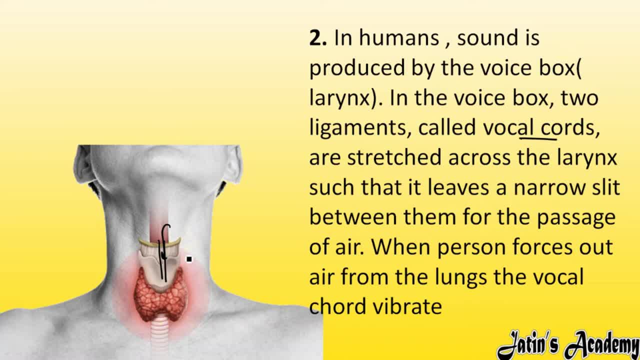 What is produced by producing vibration, Sound is produced. So, according to this, sound is also produced in humans by using the vocal cords. So what was there in the vocal cords? There was a narrow slit in the vocal cords. When the air passes through the narrow slit, 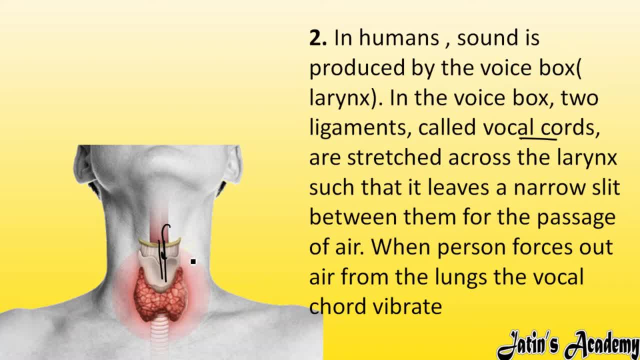 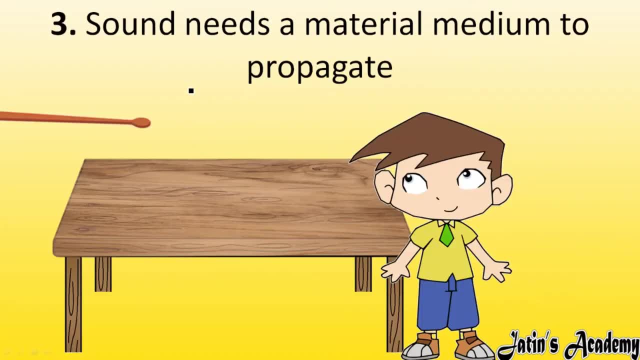 that allows the vocal cords to vibrate. And whenever the vibration will be produced, what will be produced by the vibration? Sound will be produced. So, in the same way, human beings produce sound. So next topic we are having: Sound needs a material medium to propagate. 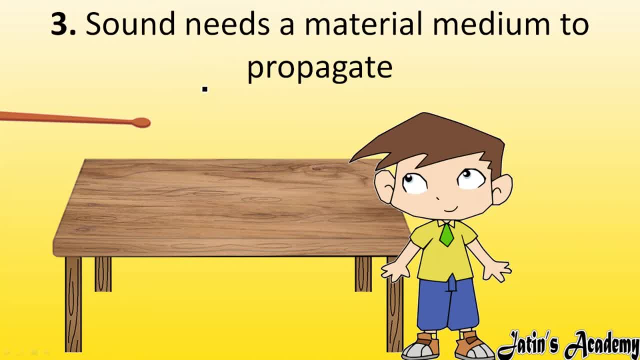 Whenever the sound has to move from one place to another, then the sound always needs a material medium. Either it needs some particles, or it needs solid particles, or it needs a liquid one, or it needs a gaseous state. Sounds always need a material medium in order to propagate. 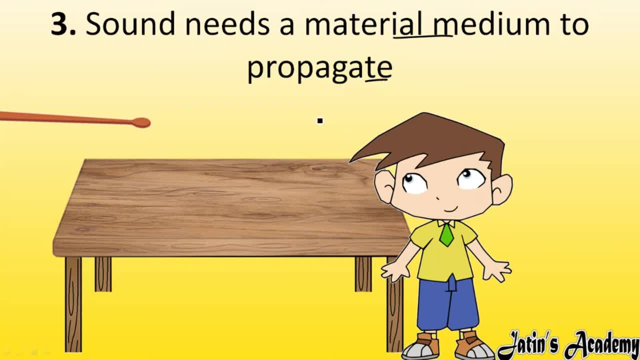 Propagate means in order to move. So I call this property of sound a mechanical wave. What is a mechanical wave? That is the property of any substance or any sound which needs a material medium to propagate, For example, be it a sound. 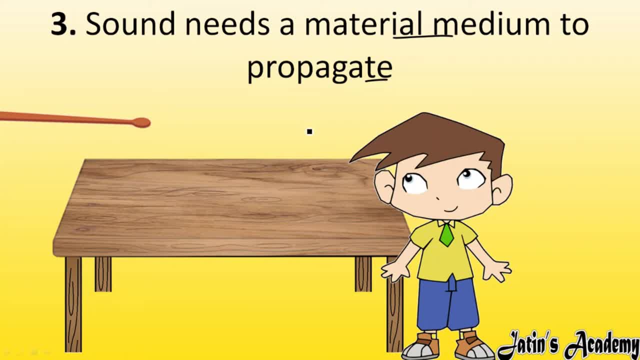 if the sound needs a material medium to propagate. This we call a mechanical wave. So what kind of sound is acting? Sound is acting as a mechanical wave, Why? Why is a sound a mechanical? Because a sound needs a material medium in order to propagate. 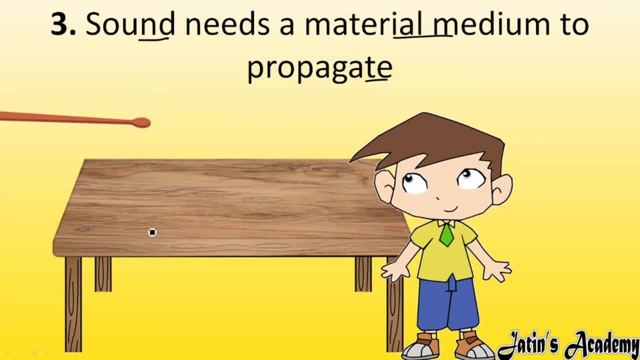 So here is an example. take a graph. I have any solid here. I strike solid to hard surface. when you strike solid to hard surface, then solid will have vibrations. means to and fro will be in particles. when there will be to and fro motion in particles, then they will produce sound. 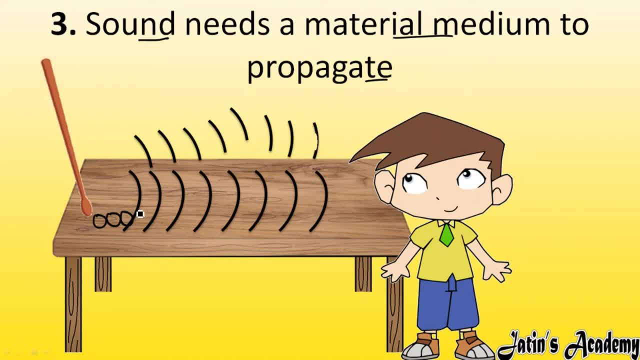 now look at the solid particles are tightly packed. when particles are tightly packed, then first particle will move to and fro, then first particle will move to and fro, then it will transfer energy to second. Now it will transfer 3rd and 4th, because particles are very close. 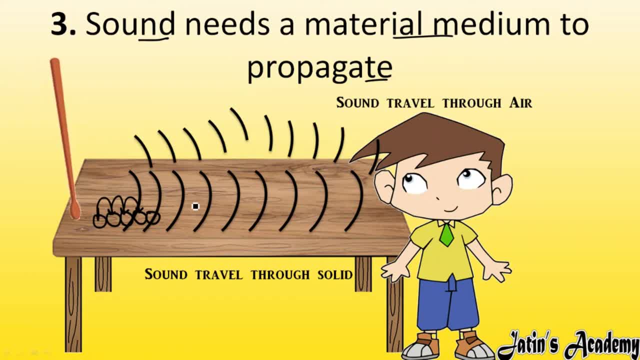 If particles are very close, then they will allow sound to move fast. So what happens is that sound travels faster in solids. So now what happened is that there are particles in solids. Very nearby particles are there Whenever we will strike these particles with a solid thing. 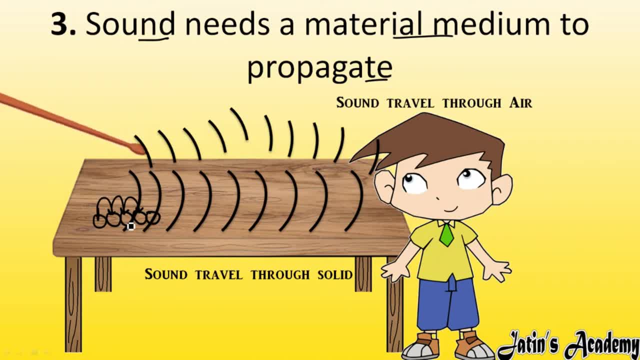 then particles will start moving to and fro motion. So what will happen is that there will be a vibration setup. If there are vibrations, then what will be produced? Sound will be produced In the same manner we are having air particles also. 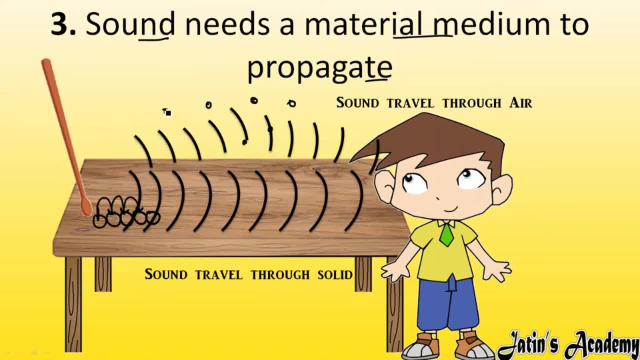 Whenever there are vibrations in air particles, Whenever we are using a speaker or anything, then what happens is that sound travels. Sound travels and makes these particles vibrate. So whenever particles vibrate, they will give energy to the next particles. Next particles will start vibrating. 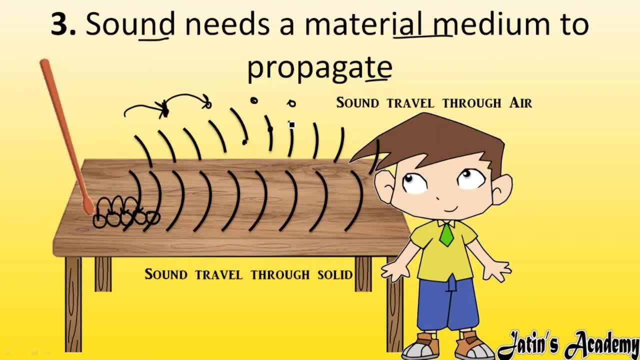 So what will happen is that sound will transfer from one place to the second place with the help of material medium. This is called mechanical wave. So sound is a mechanical wave. So in solids sound travels more faster as compared to liquid and as compared to gaseous. 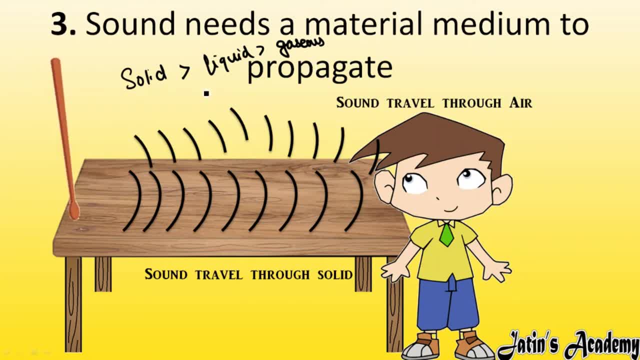 Means in gaseous state sound travels very least. Why is the answer like this? Because the particles of solids are very close. What happens when particles are close? The transfer of energy is done quickly. What are those particles? They easily transfer energy. 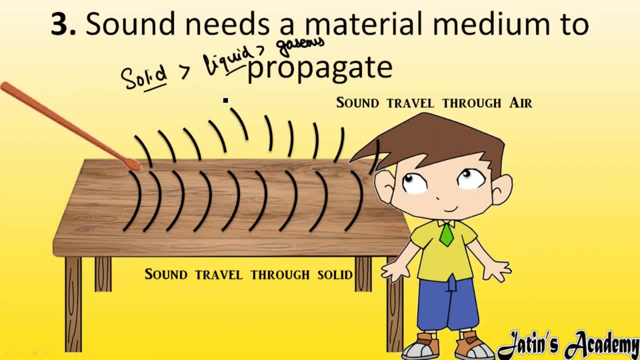 So sound propagates quickly and moves. Particles are a little far away. in liquids, When particles are far away, energy transfer is a little less, So sound is produced less in this Okay, And particles are further away in gaseous state. 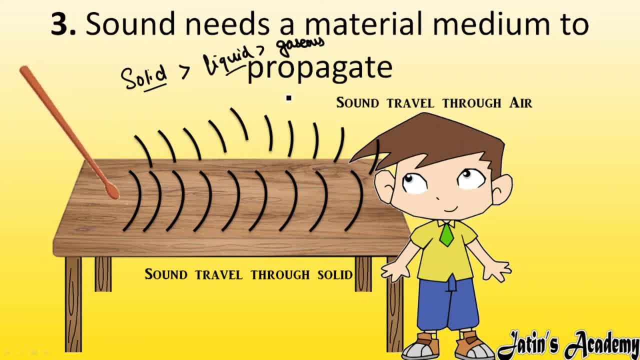 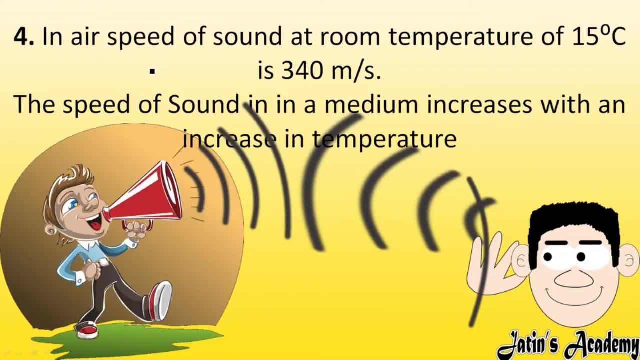 When particles are further away, the transfer of energy will also be less. If the transfer of energy is less, then the speed of sound travel in gaseous state will be slow. Okay, Next point we are having In air. the speed of sound is 340 m per second. 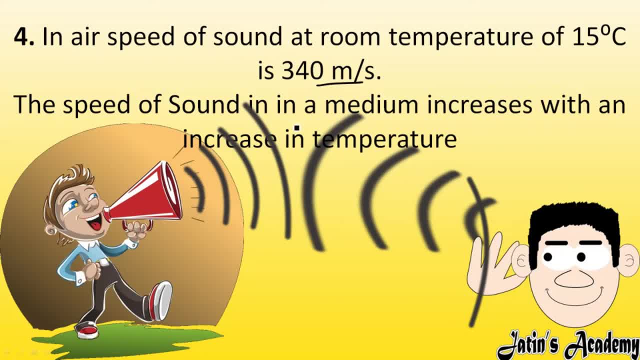 As we have read, in light energy, the speed of light is 3 x 10 to the power of 8 m per second. This is the speed of light. Now I have to find out the speed of sound. At what speed does sound move? 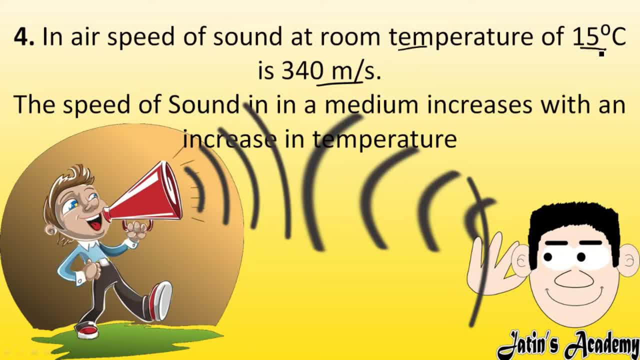 At normal room temperature of 15 degrees Celsius. In this condition, the speed of sound moves at 340 m per second. Okay, And if we increase the temperature of this atmosphere? what will happen? by increasing the temperature, The speed of sound will also increase. 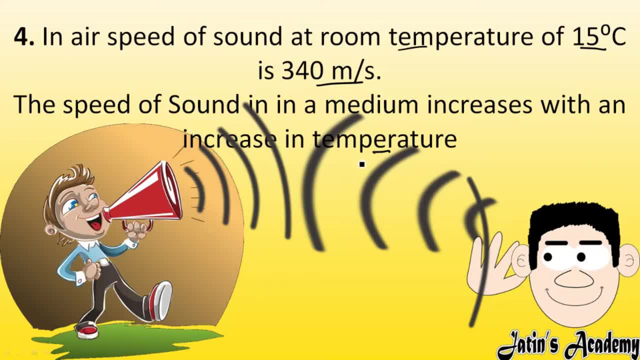 So speed of sound and temperature is directly proportional. If I increase the temperature, the speed of sound will increase. If I decrease the temperature, the speed of sound will decrease. Next we are having fifth point. In fifth point we are having sound travel. 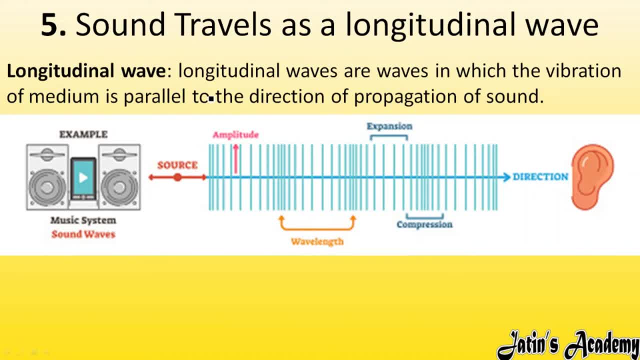 Sound travel as a longitudinal wave. When sound is produced, it travels as a longitudinal wave. Now, what is this longitudinal wave? Look carefully, What is the meaning of longitudinal wave? For example, I have taken any material And if I am striking the material with a hard surface? 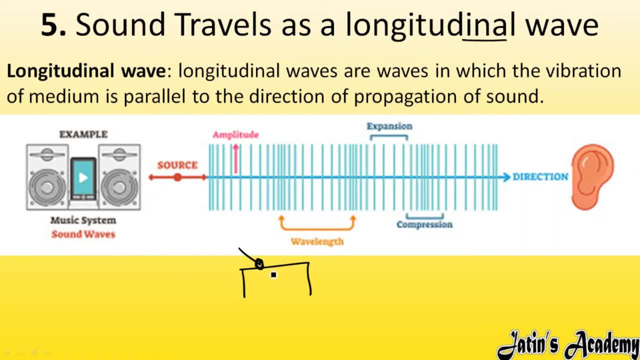 then the particles of the material are going parallel in the direction of sound. If the sound is also going in this direction and the material medium particles are also going in this direction, then the particles are also going in this direction. So if the particles are going in the parallel direction, 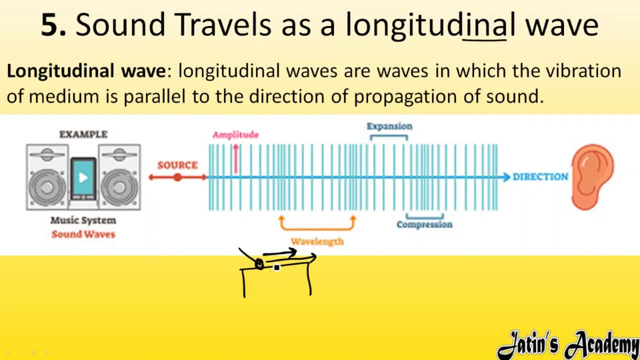 propagation of sound and material medium. particles are also vibrating in the parallel direction. Vibration means that they are vibrating like this: Okay, So if the particles are vibrating like this and the sound is also going like this, then we call it a longitudinal wave. 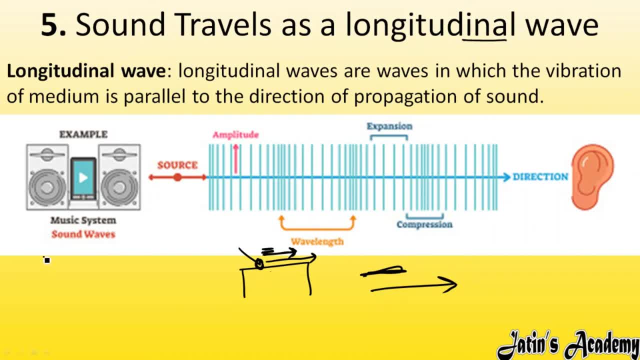 Got it. And the second we have is the transversal wave. What is the second? we have Transversal wave. So what happens in the transversal wave If I have any hard surface and I am striking it with a surface? 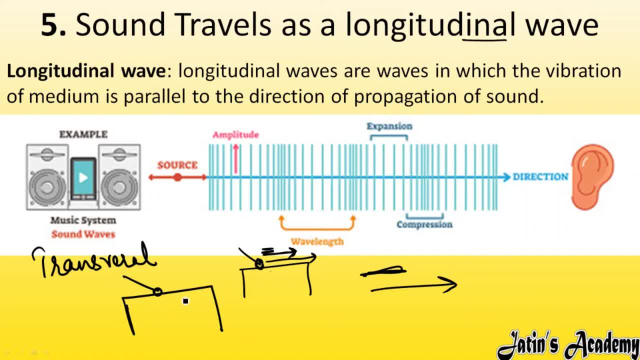 then what will happen? The particles of this surface, the particles of this surface, they will move perpendicularly, like this, And the sound will move like this: okay, The sound will move in a straight line And the particles will move perpendicularly, like this: 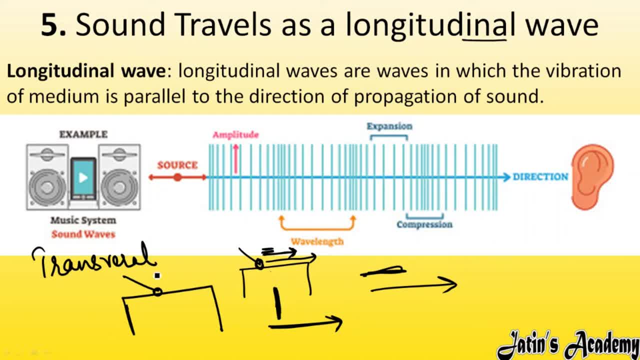 And the vibrations of the action will be like this. This is what we called as transversal wave. What was the longitudinal wave? That is, if still material medium particles are moving in this way, in the direction of propagation, of the movement of sound. 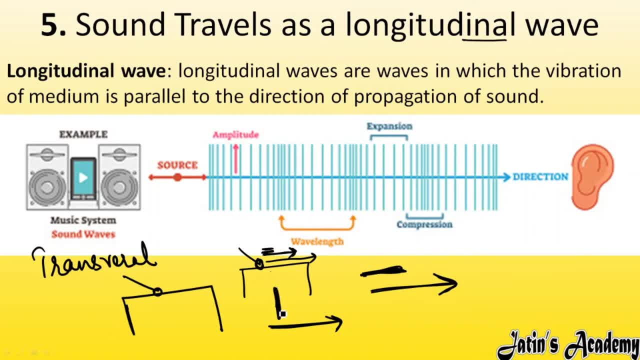 this. we call it a longitudinal wave. If the particles are moving perpendicularly in the direction of the propagation of sound, this is called transversal wave. okay, Okay, first look at the diagram of transversal wave. this is the diagram of transversal wave. 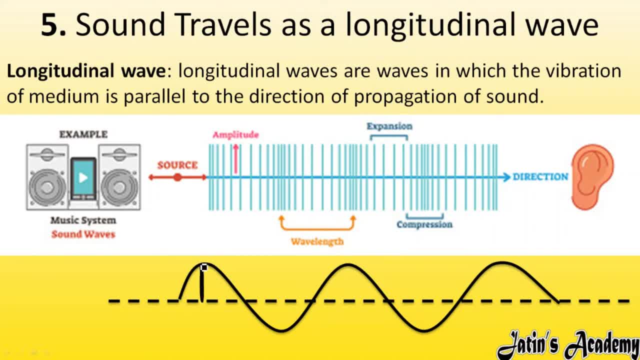 in which particles are moving in the perpendicular direction. now look at the diagram of longitudinal wave. in longitudinal wave, particles are moving like this: some particles are close to each other and some are very far away. some particles are like this: now, when particles are together, we call it compression region. 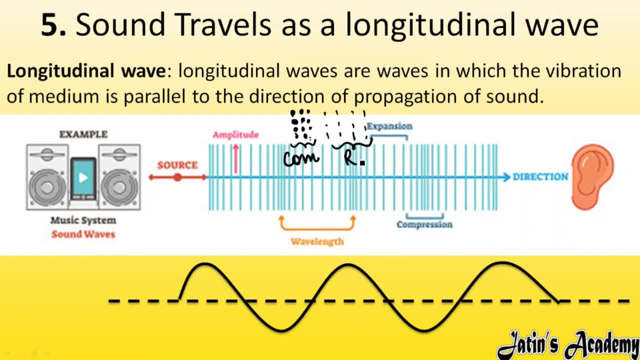 and when particles are far away, we call it rarefaction region. this is rarefaction region and the particles which are close to each other, we call it compression region. so this is the diagram of longitudinal wave and this is the diagram of transversal wave. so how to make compression and rarefaction region? 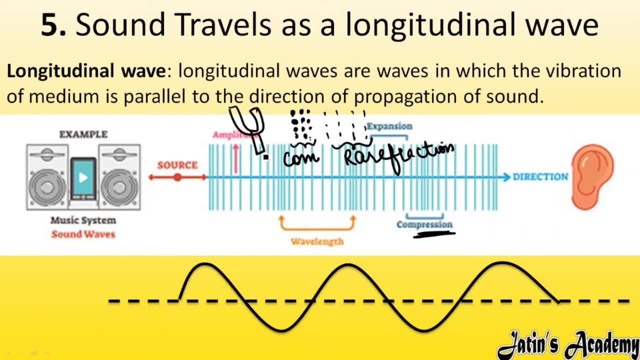 for example, i have tuning fork. tuning fork is a device which produces sound when we struck it with a hard surface. when i struck it with a hard surface, tuning fork will produce sound. so how it will produce sound, see carefully. to produce sound. first it will transfer energy to air particles. 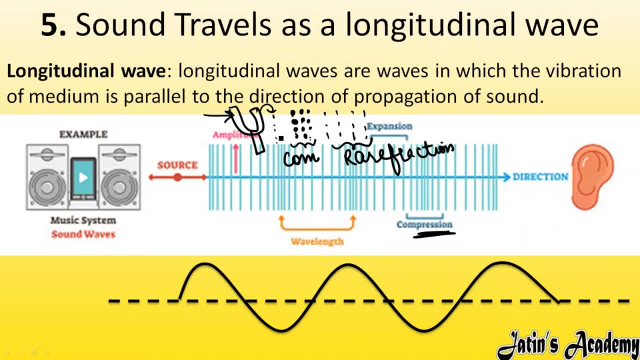 air particles will start moving in to and fro motion. when air particles will move in to and fro motion, some particles will vibrate like this. then it will transfer its energy. when it will transfer energy, particles will go far away. now the particles which i have transferred, the energy. 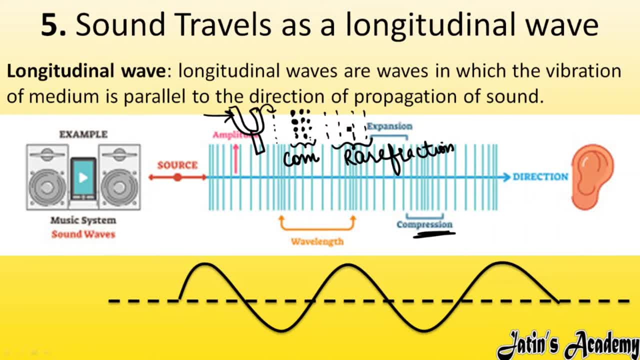 which this particles have transferred energy to the second. now those particles will come closer. so in those particles what will happen? those particles which are coming closer we will call it compression, and those particles which are going far away we will call it rarefaction region. so in longitudinal wave there is always reason for compression and rarefaction. 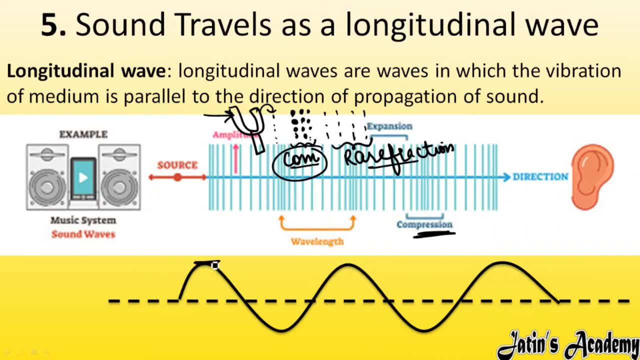 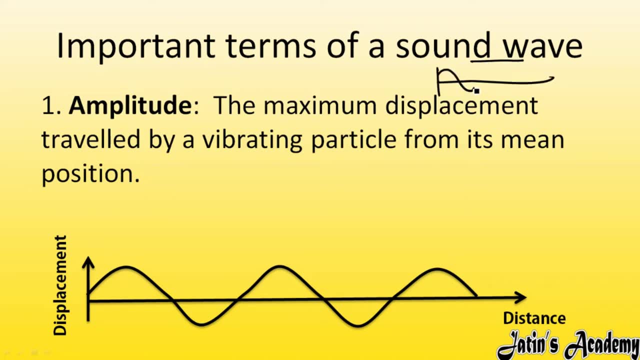 the upper line in the transversal wave is called crust. this is the crust and the downward line is called trough. upper wave is the crust, is the crust and downside wave is a trough. so next we are having some important terms related to a sound wave. sound wave. we are going to see some important terms. what are? 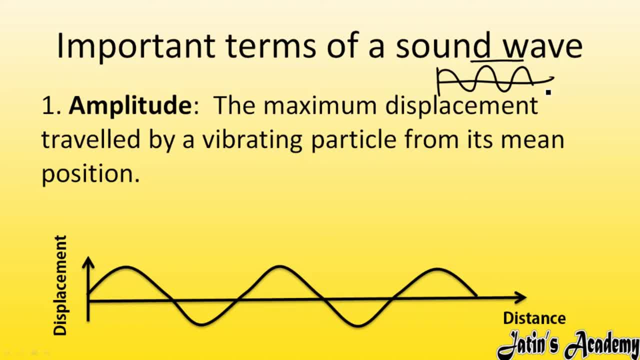 the important terms. we have a sound wave. actually it is a transversal wave. so in this chapter we will consider the whole wave, that we will study the transversal wave first. we will study what is amplitude. amplitude is the maximum displacement. how much maximum displacement? 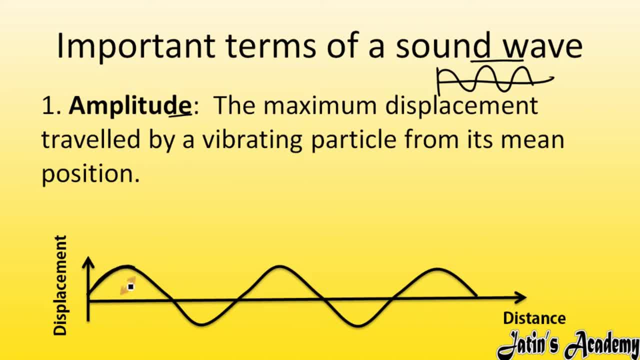 in one wave shows the maximum displacement. one wave shows how much we call amplitude. let us represent amplitude with shaking capital, with C. ok, then what is the definition? the maximum displacement travelled by a vibrating particle is to what a particle, so far, how much maximum distance show, makes. it is called amplitude from its mean position. 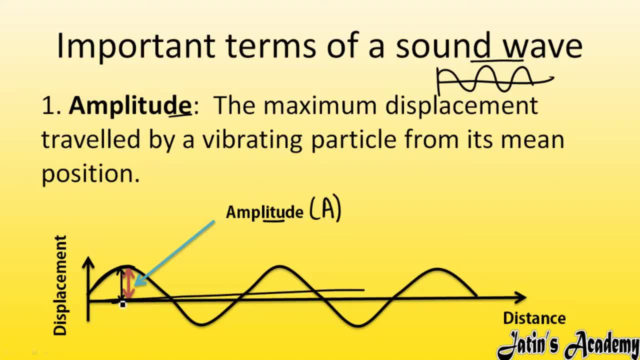 mean position is mean position only from mean to extreme. how much displacement does it show? our Obrig is called amplitude. amplitude shortcut is there to get the distance. we will take height. we addition, where you distance hai to distance ki assay unit, kya hoti hai meter. similarly, assay unit of amplitude is: 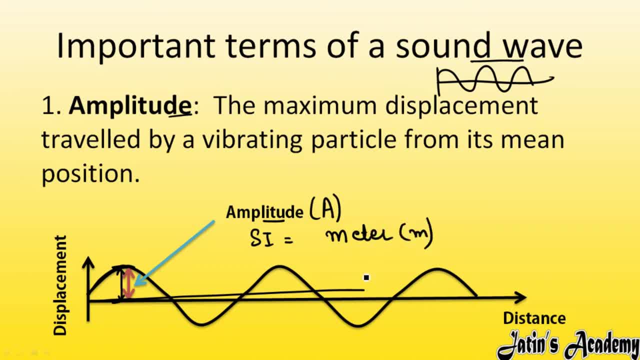 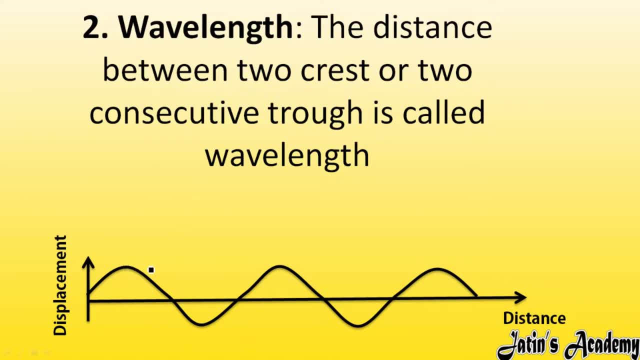 also meter, meter ko represent karenge, small mc theek hai. so next important term we are having wavelength to wavelength ka matlab. kya hota wavelength ka matlab hota distance between the two consecutive crust. consecutive ka matlab hai saath saath wali. jo distance hota saath saath wali. 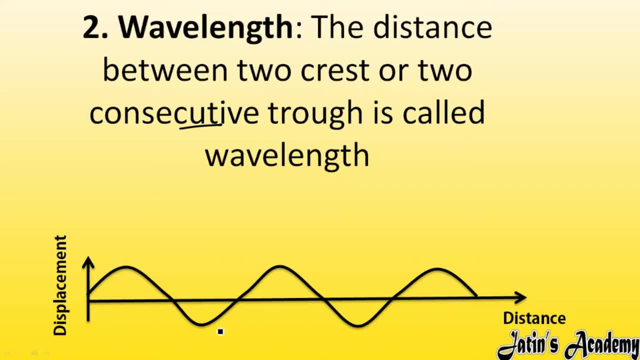 crust mein. or you can say the distance between the two consecutive trough saath saath wali, trough saath saath mai or yaha to distance between two consecutive dudea. yeah, difference between two consecutive trough ko kh doy, kya bolte hai, wavelength bolte hai. so wavelength ko represent karte. 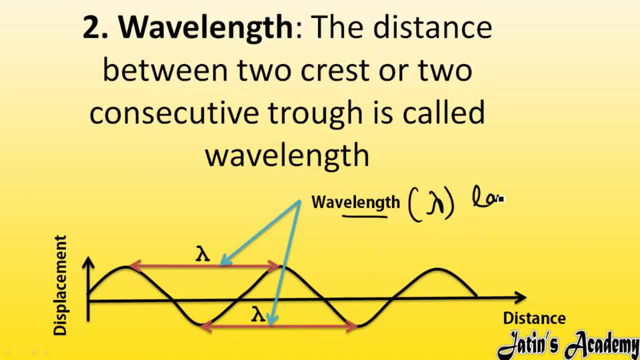 hai by the same symbol. lambda. lambda symbol hai uska, or just ka unete ve внутри. maximum distance: the distance between the two crust and distance between the consecutive trough". what is the unit of distance, meter? similarly, what is the unit of wavelength? 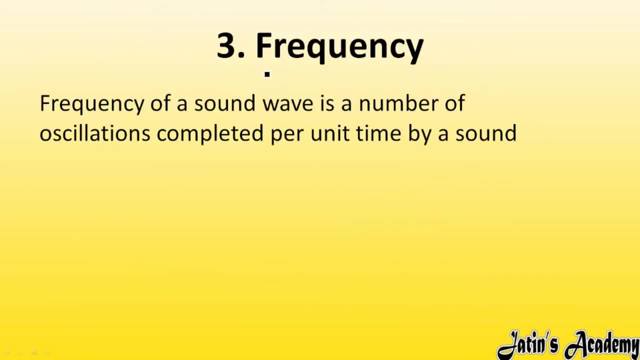 meter clear. next we are having third important term, and that third important term is frequency. so what do you mean by frequency? see carefully: frequency of the sound wave is the number of oscillations completed per unit time in one second. how much frequency does a wave have? 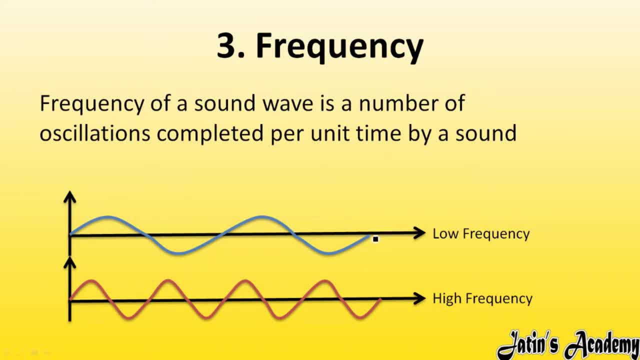 how many number of oscillations it has completed. that is called frequency. from here to here, for example, this is one second time period. from here to here, this is also one second time period. in one second time period, how many oscillations did a wave have? 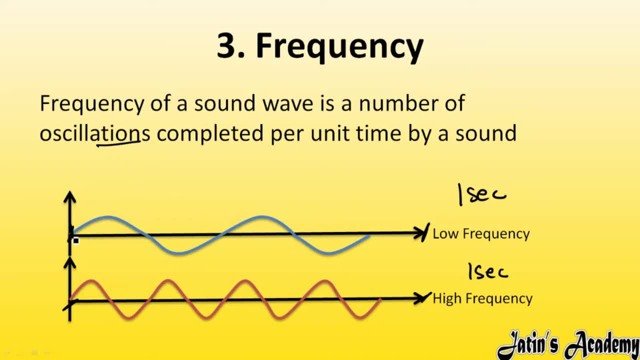 now, what are oscillations? start from here: first upper, then lower, one crust and one trough, then ok, this is one oscillation in one second. it completed only one oscillation now. start from here: one crust and one trough. how many oscillations did it show in one second? 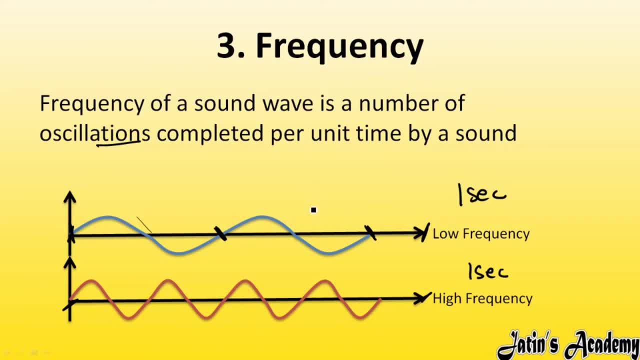 one then two. so how many oscillations did it show in per unit time? that is called frequency, so its frequency will be two, similarly, if I talk about this. so what did it do in one second? now start from here. one, then two. one crust and one trough. 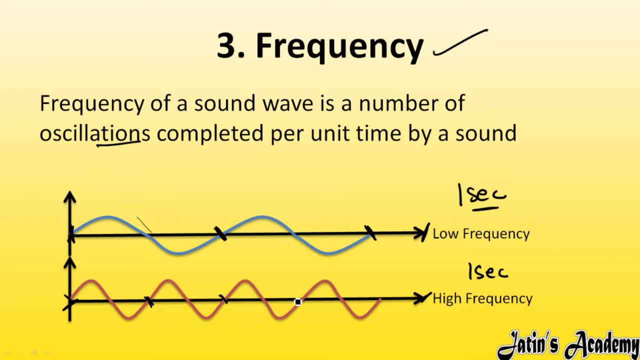 now start from here. one crust and one trough, then again one crust and one trough. so how many moves did it make? one, two, three, four. so it has oscillated four times in one second. in one second it has oscillated two times. so whose frequency is more? 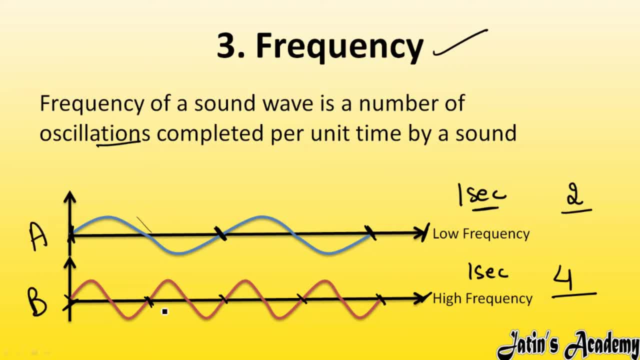 its frequency is more of B. so from A and B, B's frequency is more and A's frequency is less. frequency is understood that number of oscillations per unit time, in one time, in one second. how many number of oscillations did it complete? that is called frequency. 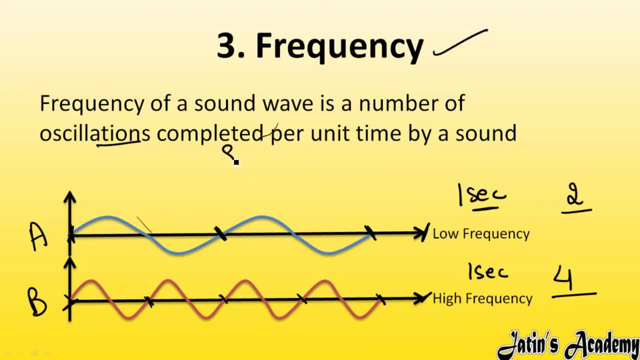 now we are having the SI unit. so what is SI unit of frequency? SI unit of frequency is hertz. hertz is the name of a scientist, scientist's name is HRhertz, so scientist's name is HRhertz, so scientist's name is HRhertz. 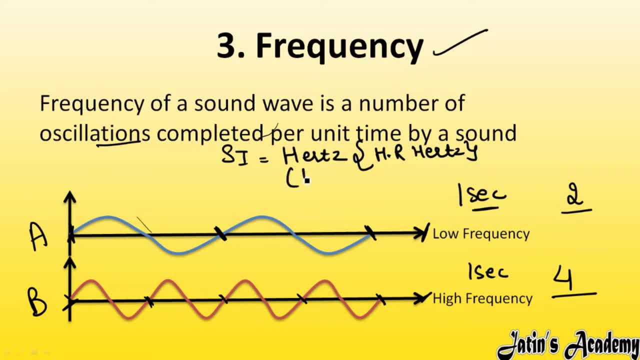 so scientist's name is HRhertz. how we will represent it? H capital, Z, small, so we will represent it like this. next, we are having symbol of frequency, so symbol of frequency is new. write the frequency like this, make V like this, so symbol of frequency is new. 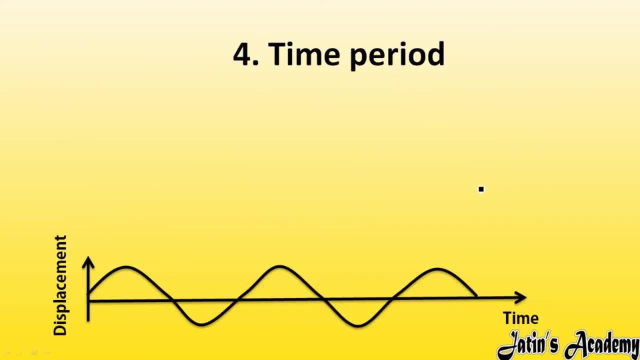 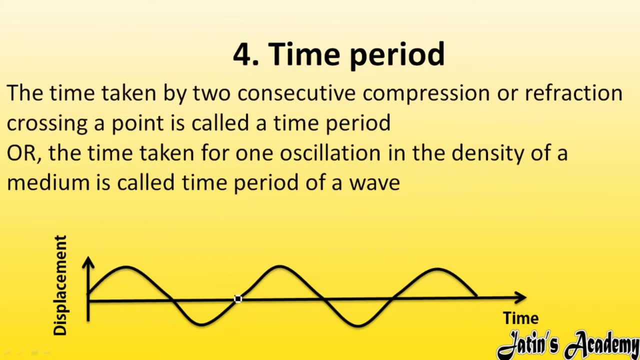 and SI unit of frequency is hertz. so next we are having time period. so what is time period? see carefully. to complete one oscillation: how much time did one wave take to complete one oscillation? how much time did one wave take? that is called time period. 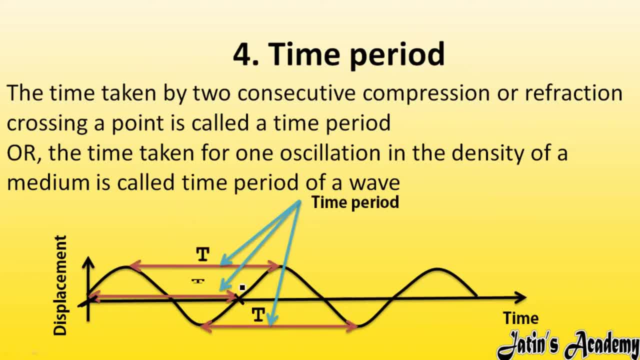 if you see from here to here, then this is also time period- to complete one oscillation. how much time period did it take? that is also time period and you can say time taken by two consecutive compression, two consecutive compression and you can say two consecutive crust- here you can write crust. 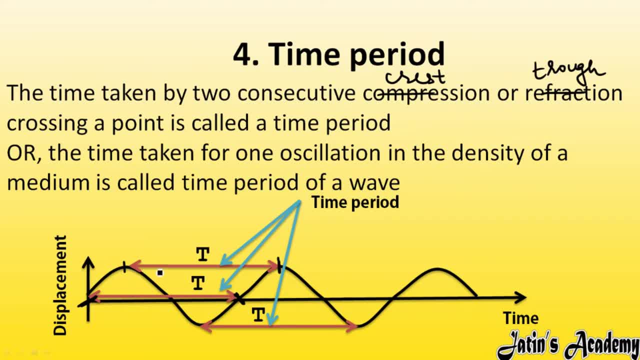 two consecutive crust and two consecutive trough and you can say time taken by two consecutive crust and time taken by two consecutive trough. that is also known as time period. or you can say time taken for one oscillation to be complete. that is known as time period of the wave. 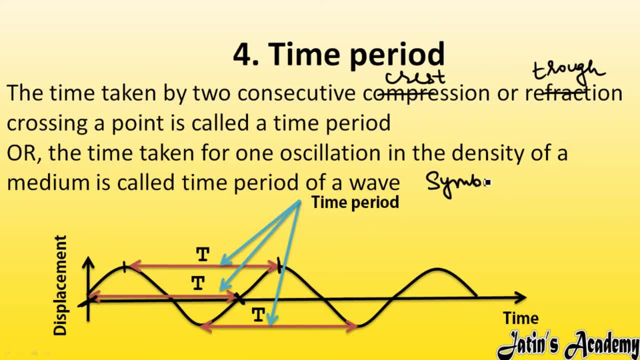 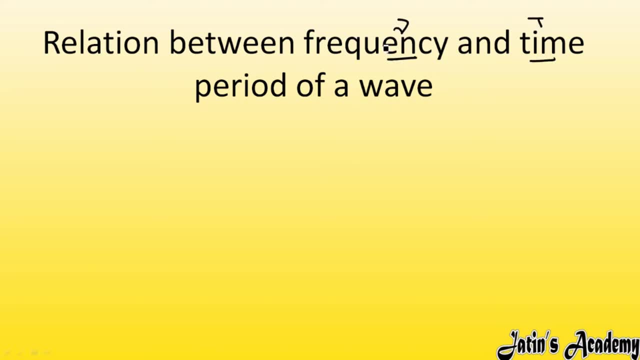 so what is time period symbol? time period symbol is capital, T, and what is SI unit of time period second. so symbol is T and SI unit is second. now we are having relation between frequency and time period- frequency is new and time period is T- and relation between frequency and time period. 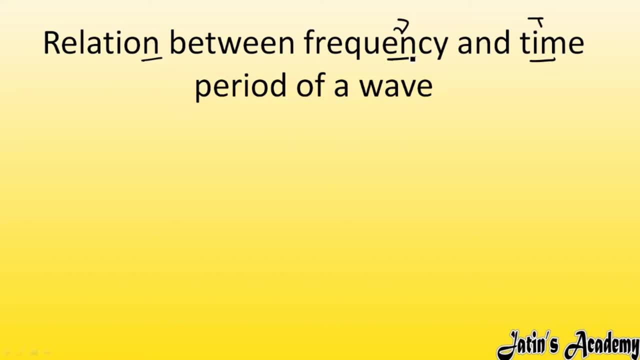 what is technology? just keep this in your mind: frequency and time period are inversely proportional. inversely proportional means frequency is equals to 1 over time period. or you can say: time period is equals to 1 over frequency. sometimes it happens in numerical if frequency given is time period. 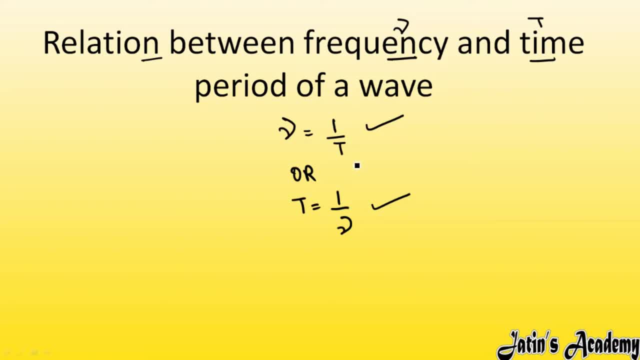 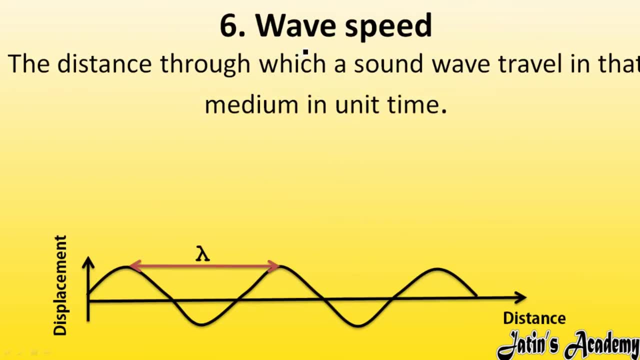 then you have to use this formula and if it comes in reverse, then you have to use this formula. frequency is equals to 1 by t. so next we are having six important term, that is wave speed. so what is the meaning of wave speed? one wave has travelled how much oscillation and how much distance. 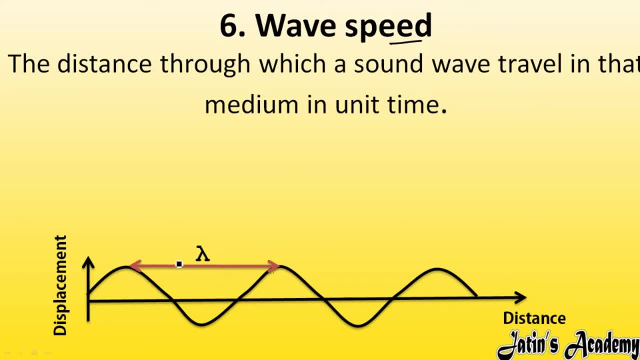 that is called wave speed. the distance through which sound wave travel in the given medium. that is how much distance travelled in sound wave in a unit time. that is called wave speed. similarly, in maths what we do is speed is equal to distance over time. that is, how much distance covered in how much time period. 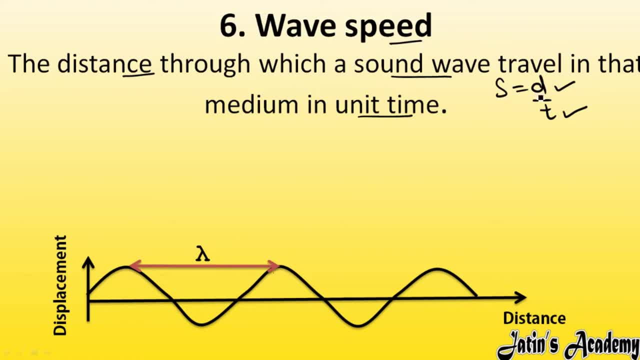 similarly, we have wave speed. so what is wave speed? distance travelled by a sound wave in the unit time that is called wave speed. what is the symbol of wave speed? wave speed symbol is v, wave speed symbol is v and its SI unit is meter per second. 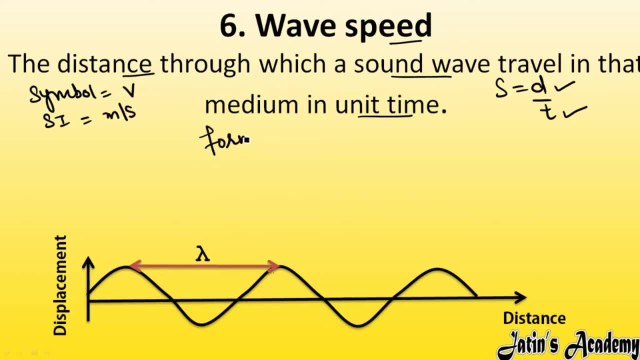 and what is the formula of wave speed? as we know, speed is equal to distance over time. we know speed is equal to distance over time. so here speed is like wave speed. v is equal to, and what is the distance? this distance is wavelength distance, that is, how much distance covered in two consecutive 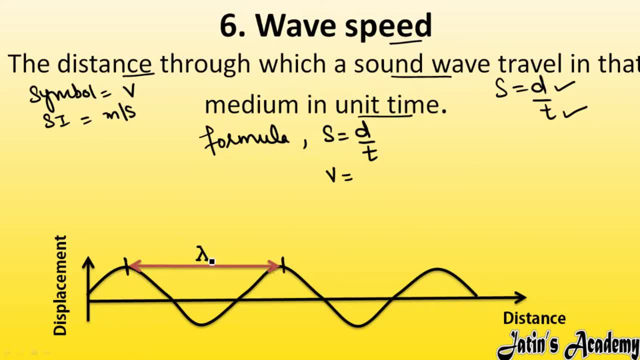 so that is how much distance covered. in two consecutive, the distance is nothing but lambda. so it will be lambda. and what is time period? time period, so it will be formula for wave speed that is lambda over, or you can say wavelength over time period. next we are having relation between wave speed, frequency and wavelength. 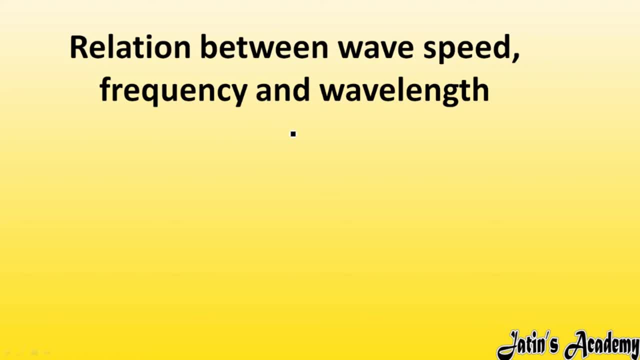 now we have taken a formula of wave speed. so what is the formula of wave speed? wave speed is equal to wavelength over time period. did you understand? now what can I do? wave speed is equal to wavelength multiply 1 over time period, because lambda multiplies 1 over time period. 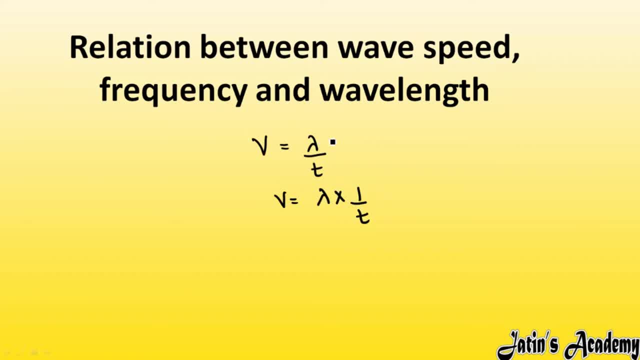 one will give you lambda only wavelength. multiply one will give you wavelength only so one by time. one by time means we just found out that one by time is equal to frequency. frequency and time period are inversely proportional, so one by time period is equal to frequency. 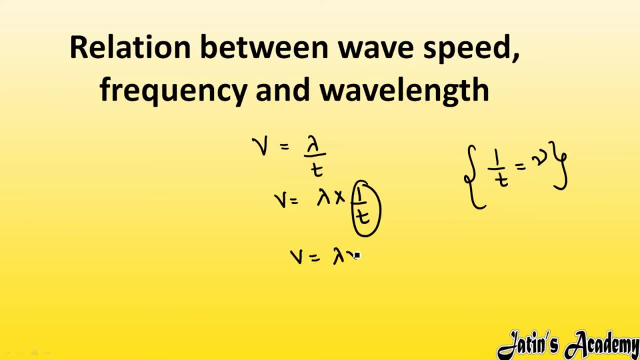 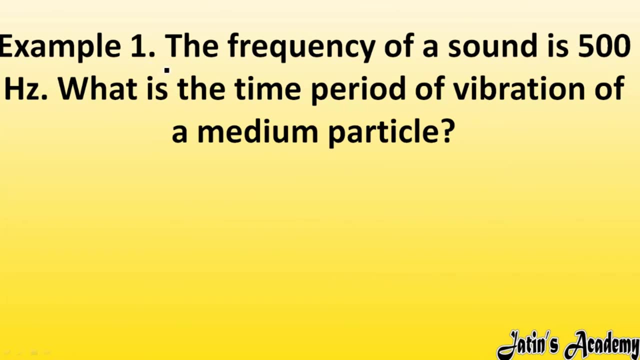 so what you do, wave speed is equal to lambda. multiply one by t, place new, that is frequency. so this relation came to me in wave speed, wavelength and frequency. this is the relation between wave speed, frequency and wavelength. okay, so now we are having some numericals related to the sound chapter. very first numerical we are having: the frequency of the sound is. 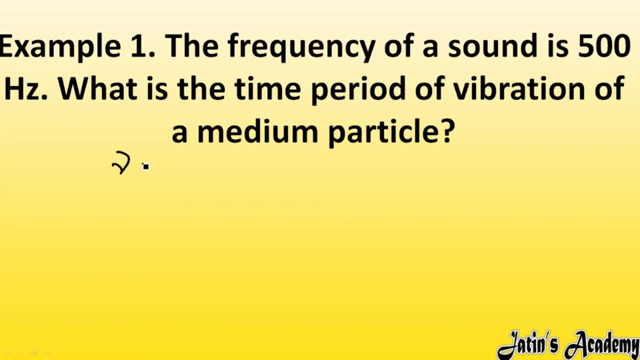 500 hertz. i have here frequency given, new given 500 hertz. what is the time period? time period will be of vibration of a medium particle, means we have to find out the time period. or you can represent time period in capital t or small t, no problem. so what we have to 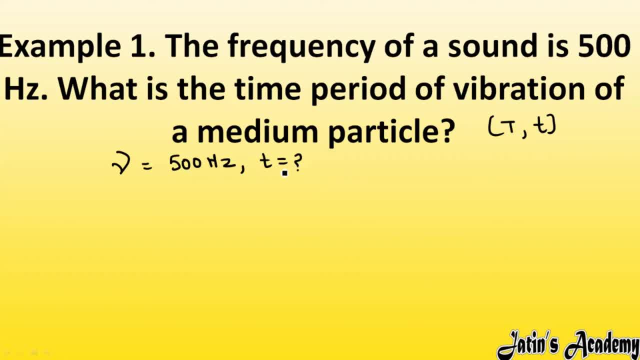 do frequency given and time period? we know what is the relation between time period and frequency. so what is the relation between time period and frequency? they are inversely proportional to each other. time period is equal to one by frequency. they are inversely proportional to each other. so what is the time period? time period is equal to one over 500, so solve. 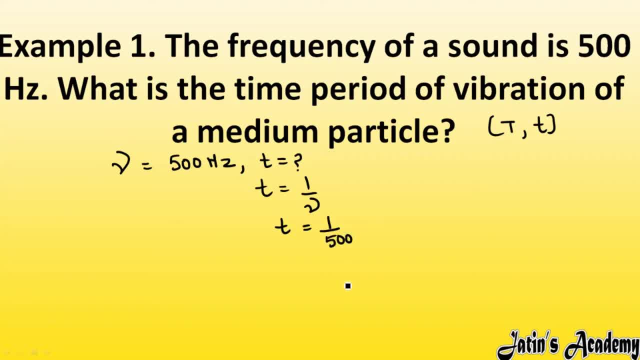 one over five hundred, it will be what to do. start dividing it, keep the denominator out, keep the numerator inside. okay, so in 500, one is not going, so put zero point. put zero point now. in five hundred the ten doesn't go, so put one more zero. one more zero then. 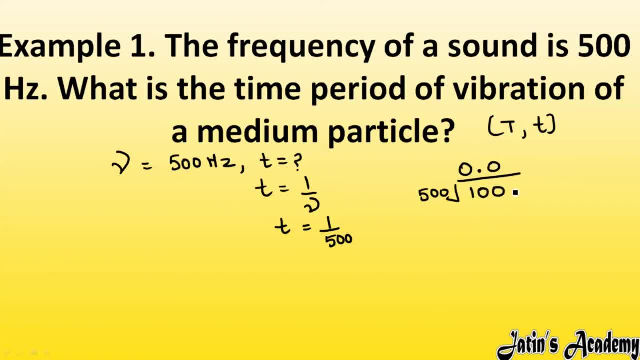 again one zero, again one zero. five hundred is the same. 1000 is equal to 1000, one is equal to 1000 and this one is equal to one because half of it- we will not know how many thousand thousand- where it goes to two. so how much will it go? it will be 0.002 second. so this is the answer. 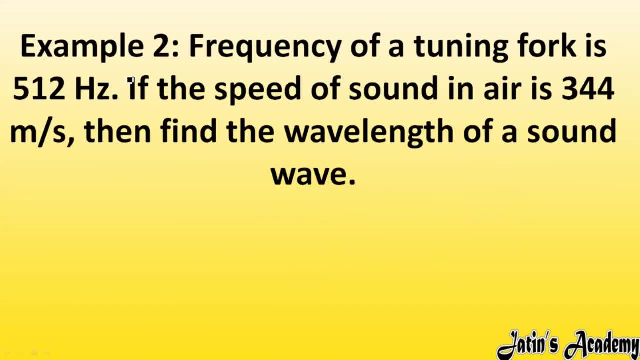 we have of time period. okay. next we're having second example. so second example we are given with frequency of tuning fork is 512 hertz. i have here frequency given. frequency is equals to 512 hertz if the speed of sound in air is this much. if i have here speed of sound given, i mean i have 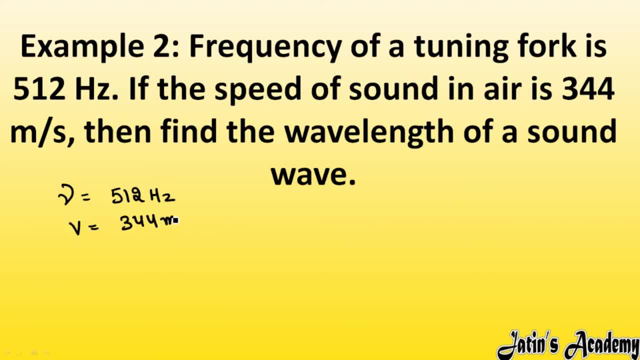 here v value given, that is 344 meter per second. then find the value of wavelength. i have to find out the value of wavelength. i have just seen the relation in wave speed, frequency and lambda. that is, wave speed is equals to lambda multiply frequency. this relation is wave speed, lambda. 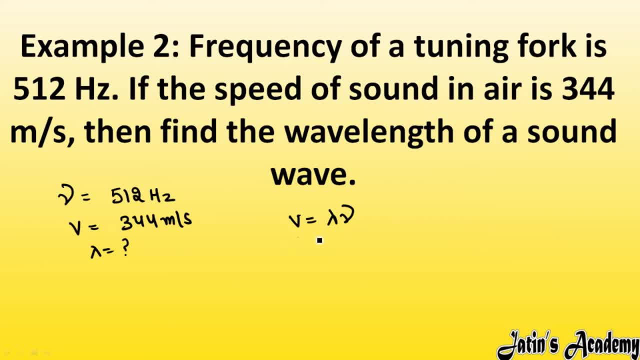 you can say wavelength and frequency. put values in this, wave speed is 344, is equals to lambda- i have to find out. and frequency is 512. so 512 here plus here divide it will be 344 and over 512 is equals to lambda. solve it: how much will it be? it will be 0.67, equals to lambda, and 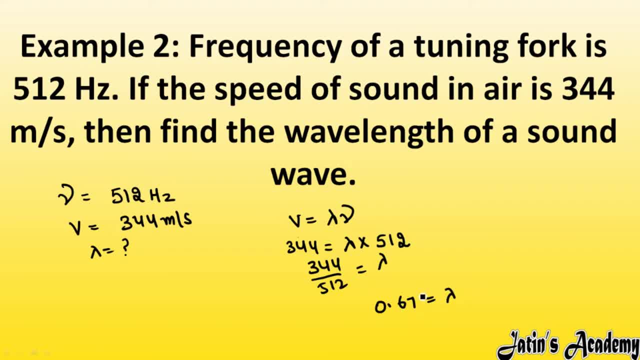 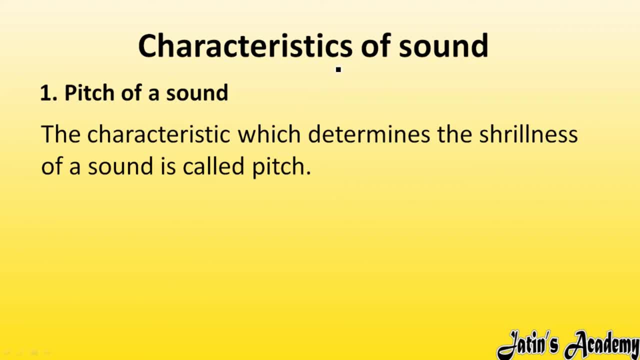 write the unit of lambda. what is the unit of lambda meter? so 0.67 meter is the answer. so mainly in this chapter we are going to read three characteristics of sound. what are the three characteristics? first we have pitch, then we are having loudness. okay, then we are having loudness. 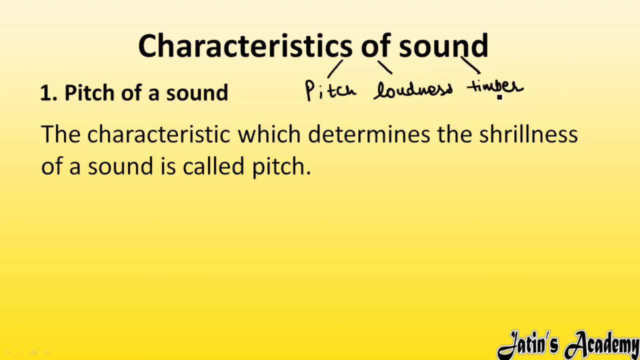 and then we are having timber, timber. you can say quality of sound. so three characteristics we are going to study here. very first characteristic: we are having pitch of a sound. so what is the pitch of sound then? pitch of sound, is that characteristic of sound that tells that our voice is so shrill, or 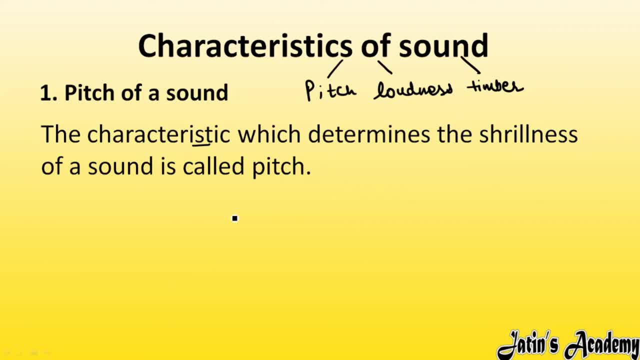 how sharp? how sharp means how sharp, deep it remains as my voice is, anyone's voice, any sound that, how scary is that sound? or how broad, how big it is. ensch, Cruelness, mining sound and broadness of sound to determine the meaning I use. which characteristic I? use pitch pitch ofização someone's voice or anyone's sound, how sharp and how heavy a sound is, how big it is, which 제�ullah me use in me. use pitch pitch of sound, as you no need to use pitch pitch of your voice. what amount much sound is in this? why the pitch is so sharp and sound? all these sounds is 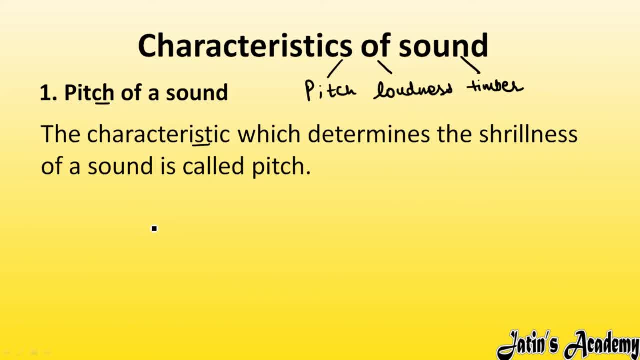 or any sound is how much stronger and how much heavier. We call that pitch of a sound clear. Now we are having a wave graph for the pitch of the sound. If the number of oscillations is more in the particular time Means it's same time period. 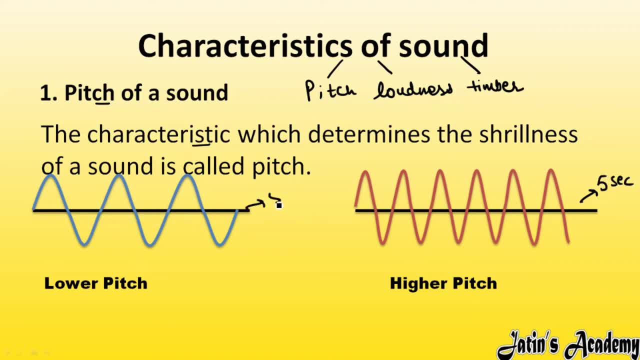 For example, this is also time period of 5 seconds and this is also time period of 5 seconds. So if number of oscillations are more in the same time period, Number of oscillations will increase. the pitch Pitch higher means the sound will be stronger. 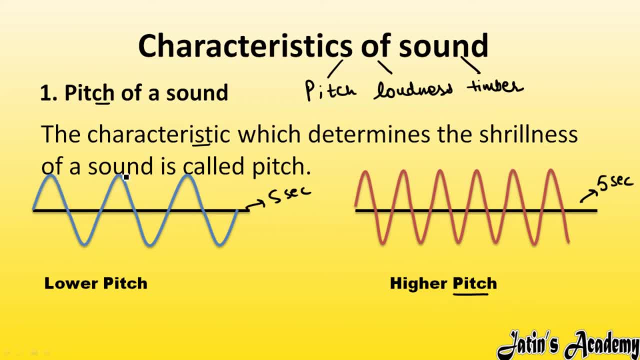 In the same time period, the number of oscillations is less. Number of oscillations is less means lower pitch. Lower pitch means its sound will be heavy. So higher pitch means shrill sound and lower pitch means hoarse sound. Hoarse sound means broad sound. 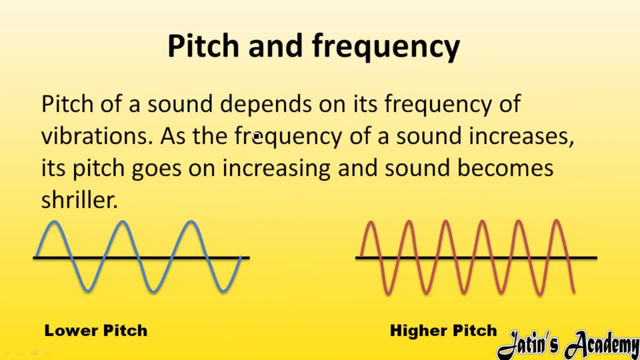 Or you can say broad, sound, Clear. Next we are having pitch and frequency. Which pitch is bent? Pitch is bent by frequency. You can see from the waves that if the number of oscillations is more means frequency is more in per unit time. 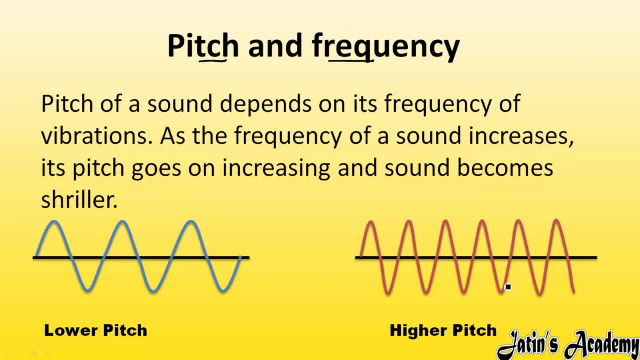 if the number of oscillations is more and you can say frequency is more, then the pitch will be higher. If the frequency is less and you can say number of oscillations is less, then the pitch will be lower. So here, higher the frequency, higher the pitch. 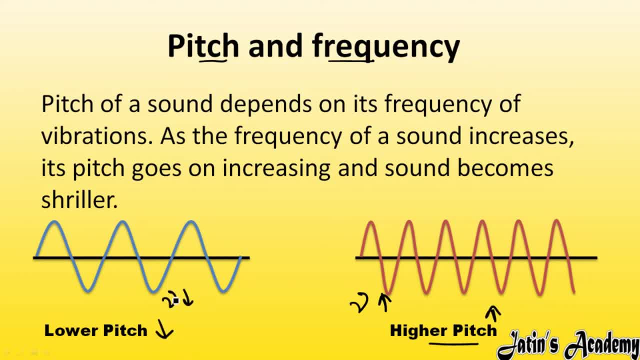 And lower the frequency, lower is the pitch, So pitch and frequency are directly proportional to each other. Clear, As the frequency increases, the pitch increases Means the sound will be shrill, And if the frequency is low, then the sound is lower pitch. 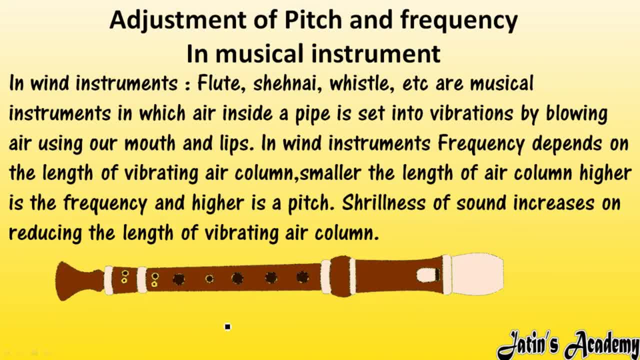 Lower pitch Means the sound will be heavy. Okay, Next we are having adjustment of pitch and frequency in musical instruments. How do we adjust pitch and frequency in musical instruments? First musical instrument we are going to study is wind instrument. So what is wind instrument? 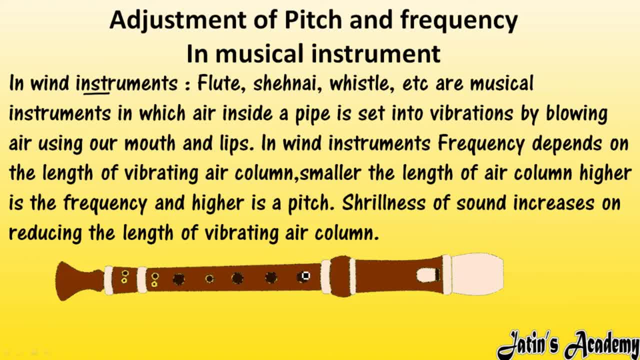 Like flute, shehnai, whistle- All these are wind instruments. All these are wind instruments. So what happens in this? There are some holes. Whenever we do in holes, if we do from our mouth or our lips, we will fill the air inside. 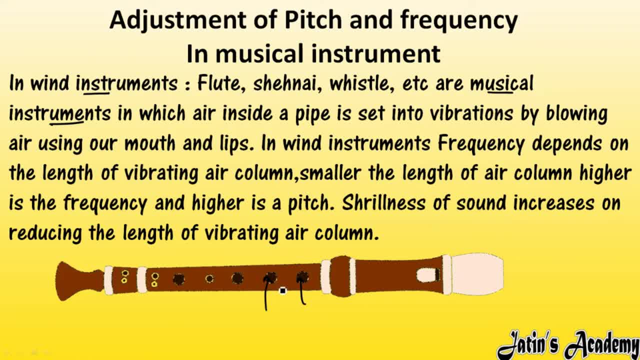 So the air particles inside vibrates. We will send the air inside through these holes. So, after sending the air, what will happen? It will be hollow inside. The flute, or shehnai is hollow inside. Hollow means there are air particles in it. 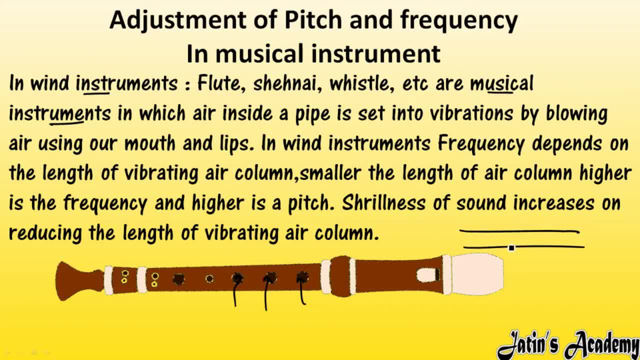 So whenever we send air through this hole with the help of our mouth. so what happens? when we send air, The air particles inside will vibrate. And when the particles inside vibrate, what will they produce? Sound pressure, So the sound will be heard. 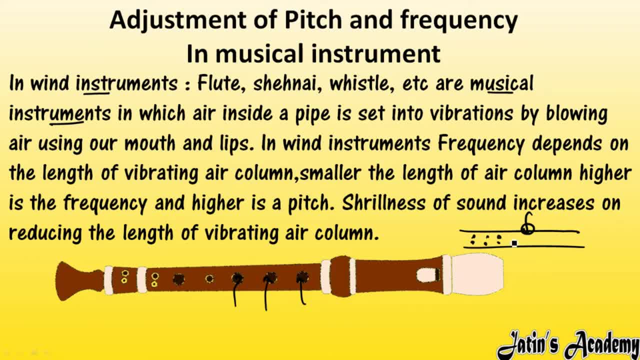 So the sound will be heard, Sound will be produced. So such wind instruments work, And the frequency in the wind instrument depends on the length of the vibrating air column. If I take the length of the vibrating air column small, then what will happen in it? 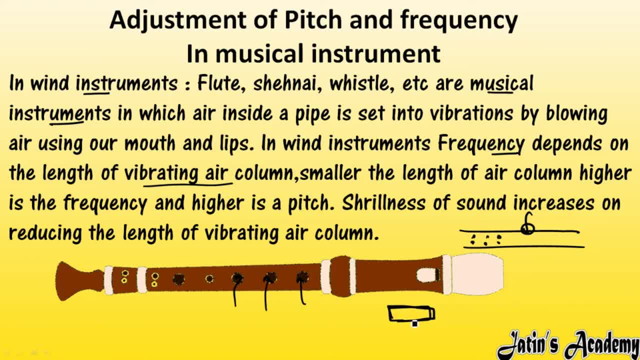 There will be a higher frequency. What will be the frequency in it If I am using a small length wind instrument, small length means higher frequency. If there is a higher frequency then its pitch will also be higher Means if I use a small length wind instrument. 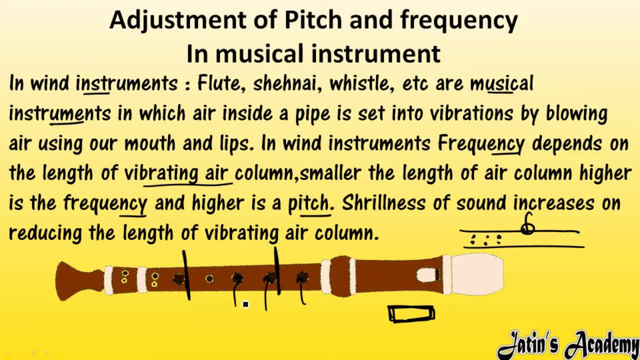 there will be a shrill sound in it. Shrill means there will be a sharp sound And if I use a long length wind instrument, If I use a long length wind instrument, there will be a higher frequency in it. There will be a higher frequency in it. 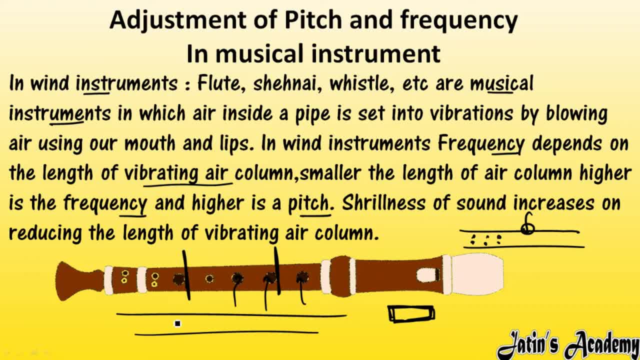 Means there will be a lower pitch in it. If the pitch is low, then the sound in it will be heavier. There will be a broad and hoarse sound in it. So we are given here that the shrillness of sound, the sound that is sharp. 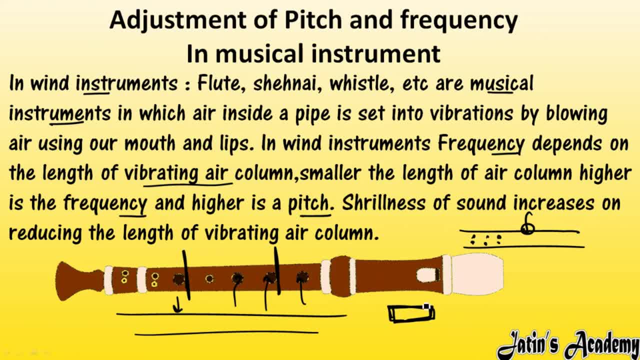 how will it increase If I reduce the length of the vibrating air column? what will I do If I reduce the length of the vibrating air column? then the sound will be shrill. If I increase the length of the vibrating air column. 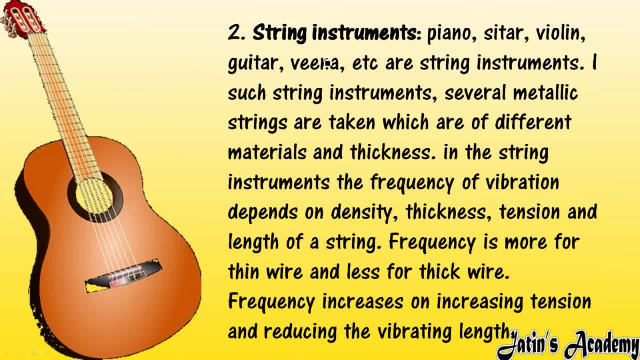 then the sound will be hoarse and broad. So next type of musical instrument: we are having string instruments. See how we adjust the frequency and pitch in string instruments First. what are the examples of string instruments Like piano, sitar, violin, guitar. 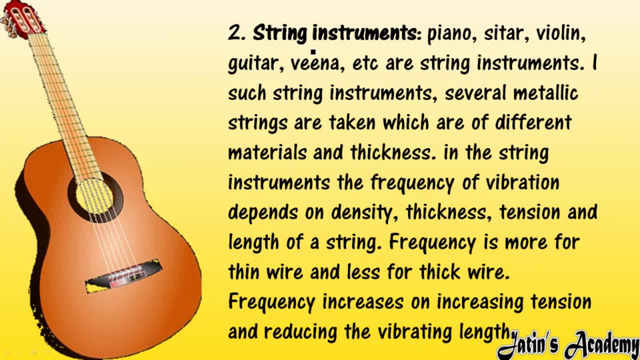 veena. these all are the examples of string instruments, Like the name itself is clear, as string. What will string mean? There will be strings in these instruments. There will be wires like this, So we call it string instrument. What are string instruments? 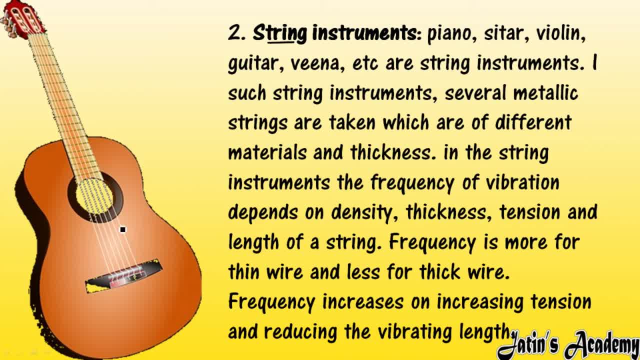 There are some metallic strings of different material and thickness. These strings are of different material and thickness. Some will be thicker, some thinner. So what happen in string instruments? The frequency of sound depends on the density, thickness, tension and length of a string. 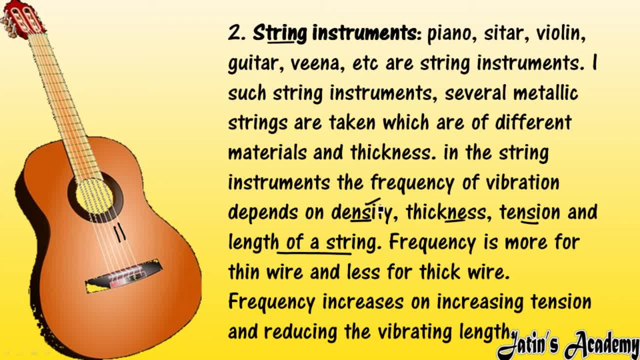 How can we change the frequency of a string? If I increase the density of the string or decrease the thickness and tension, or increase or decrease the length of the string, then only frequency can be changed. if i am taking length of thin wire, for example, i have taken thin wire. 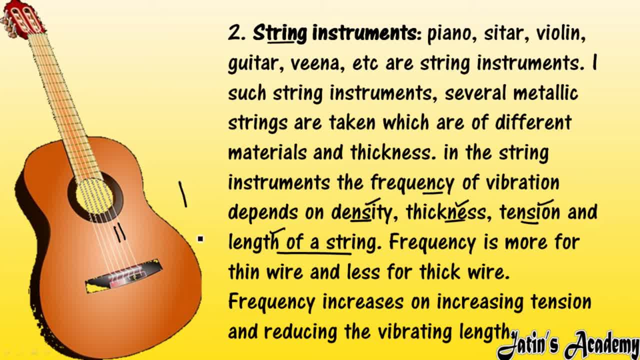 so in thin wire its frequency will be more produced, more frequency. produced means more pitch sound will come. more pitch means shriller sound will come for the thin wire. and if i take thick wire, so in thick wire the frequency will be less. frequency less means pitch less. 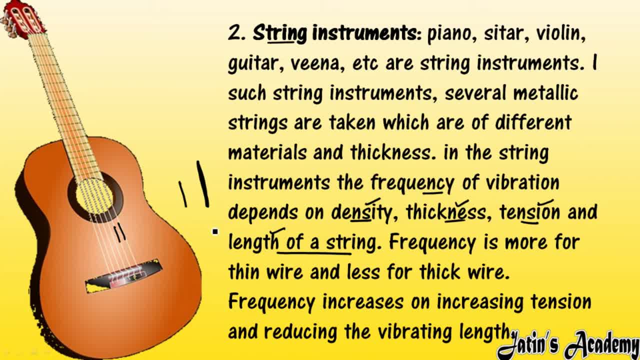 pitch less means the sound will be broad and you can say from string instrument. so when frequency increases, if i have to increase the frequency, so second way we have is to increase or decrease the frequency by increasing or decreasing the tension. if i increase or decrease the tightness of the string, 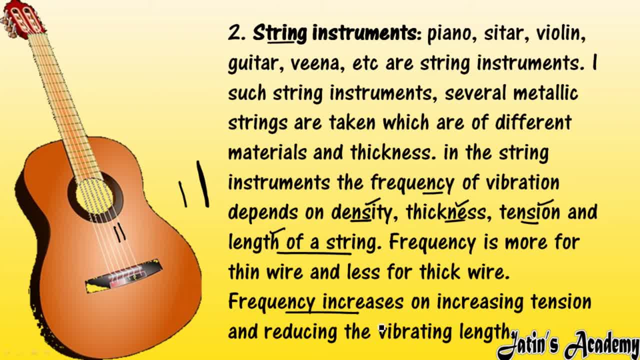 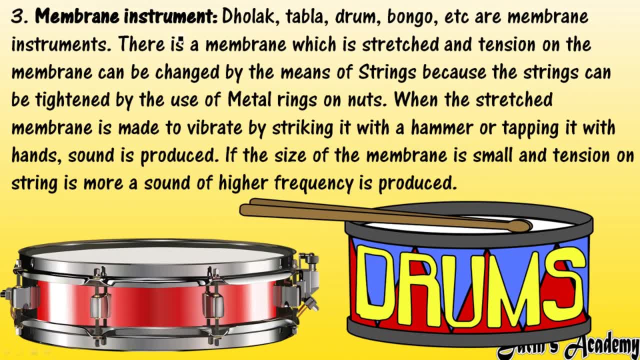 so to increase or decrease the tightness of the string, frequency will increase or decrease. so next we are having membrane instrument. so what are membrane instruments like drum, drum, bongo, these all are the membrane instruments. and what is membrane instrument? here a stretched membrane is applied. 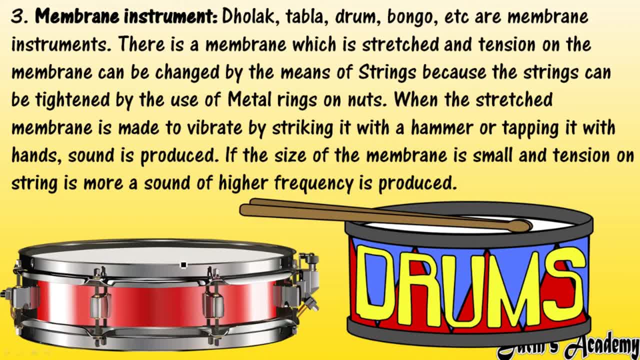 here a stretched membrane is applied and its tension of membrane. we can increase or decrease tightness of that membrane. we can increase or decrease by the means of strings. here some strings are applied. with the help of these strings i can increase or decrease the tension of membrane. 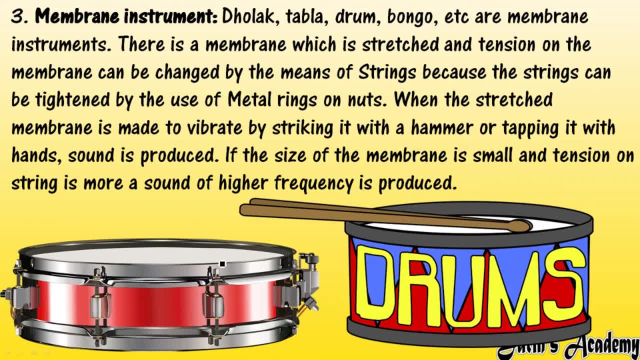 i can increase or decrease the tightness, so how i can increase or decrease the tension, which are metal rings, so i can stretch loose or tight by using these metal rings. and when i am doing this stretched membrane, what i do is when i try any hard surface. 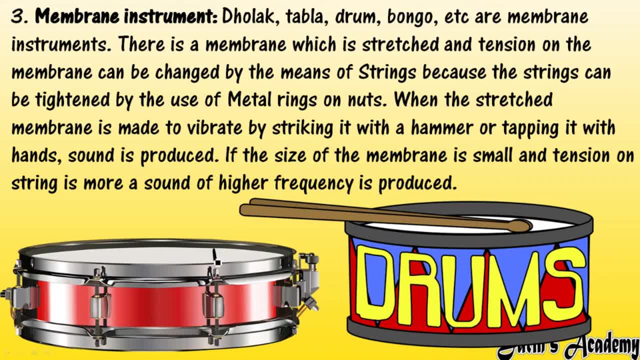 so what happens? when i try hard surface, this membrane starts to move to and fro. and when any thing moves to and fro, it vibrates. so when i tap it with any hammer, membrane will vibrate and by vibrating sound will be produced. and if the size of membrane is small, 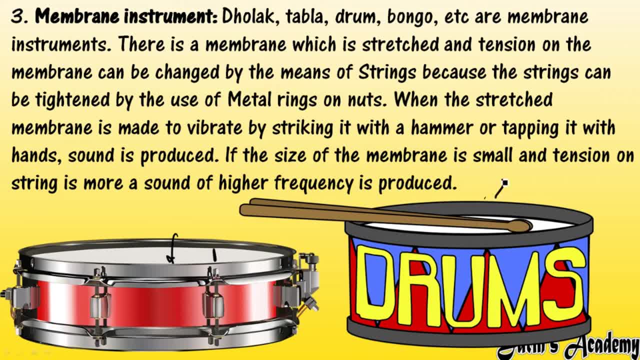 if the size of membrane is small, for example. in this case, size of membrane is small. so what will happen in that? and if the tension of string is high, sound will be produced. small the membrane, or you can say higher the tension. in this frequency, more sound will be produced. 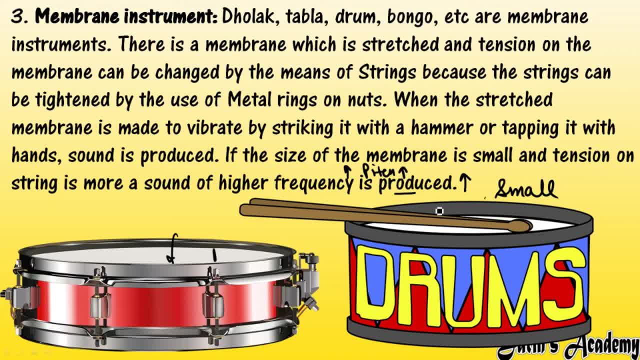 frequency means more pitch. pitch means more shriller sound. so here shriller sound will be produced and inverse, if we are having the more area membrane, if there is more area membrane and tension will be less, then here broad or hoarse and you can say heavy sound will be produced. 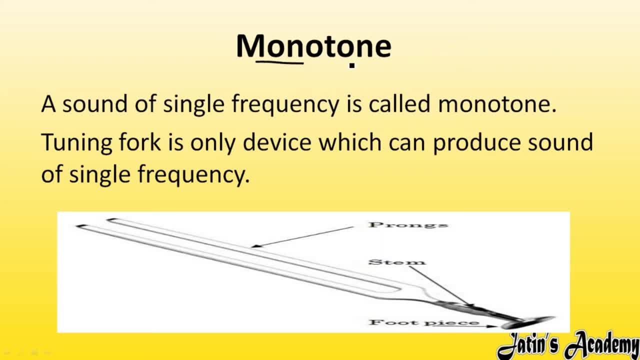 so next we are having mono tone. mono tone means mono means single, tone means single frequency. single frequency means if i say like, this sound of single frequency is called mono tone. so did you understand? did you enjoy it? if i increase or decrease my pitch, if i increase or decrease my pitch, 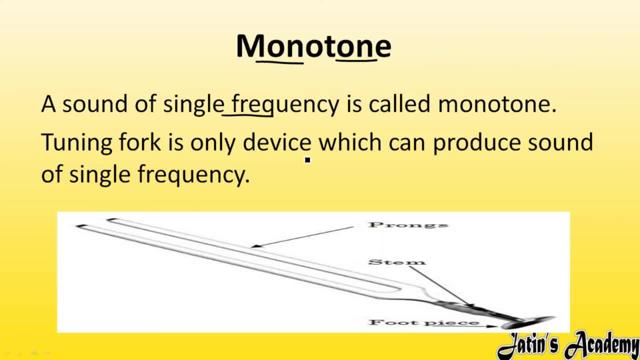 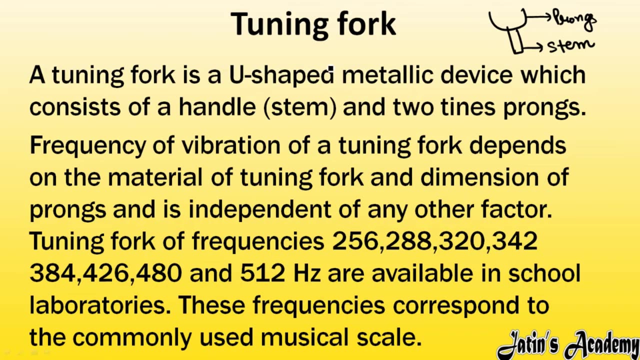 if i increase or decrease my pitch, then it will be good for listeners, so this is called mono tone. if i am speaking in single frequency, then it is called mono tone and tuning fork. this is tuning fork. tuning fork produces single frequency. so next we will study about tuning fork. 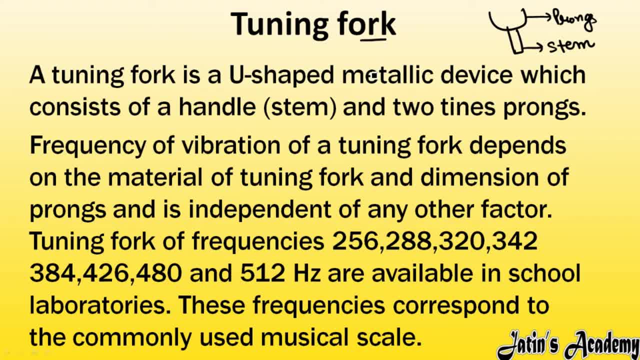 tuning fork produces monodone sound. so what is tuning fork? tuning fork is a u shaped metallic device in which there is a handle and you can say stem and two times prongs, and this is called prongs. one prongs, second prongs, this is called prongs. 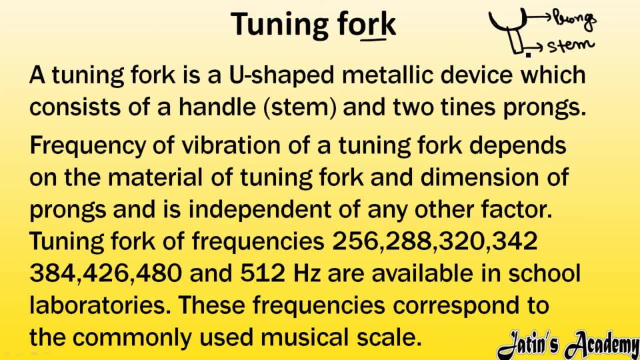 and this handle is called stem. frequency of vibration of tuning fork depends on material of tuning fork. material of tuning fork is material of tuning fork and on how material is material of tuning fork and also on dimensions of prongs. that dimensions of prongs. if dimensions are very less. 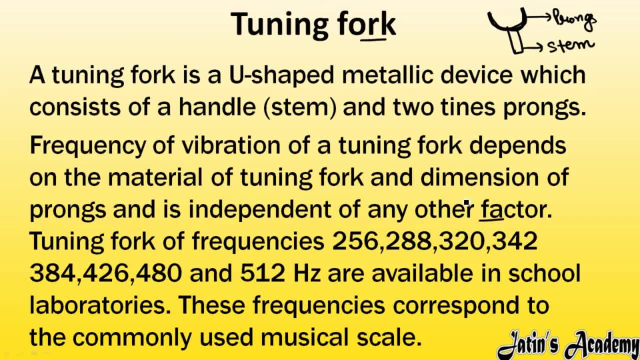 than frequency depends on prongs and frequency is depended on prongs, material of tuning fork and seconds depend on dimensions of prongs and then we will get tuning fork frequency like this. their frequency was this: we can see this easily and we use in school lab and these frequencies are: 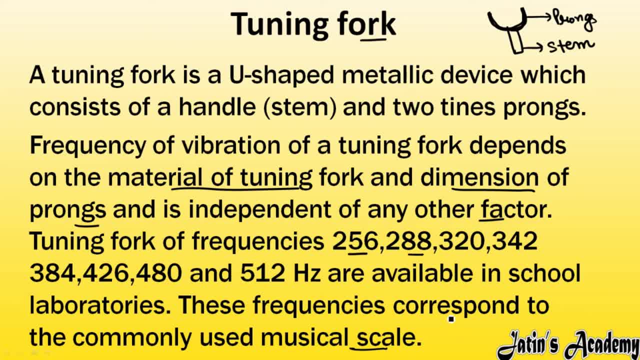 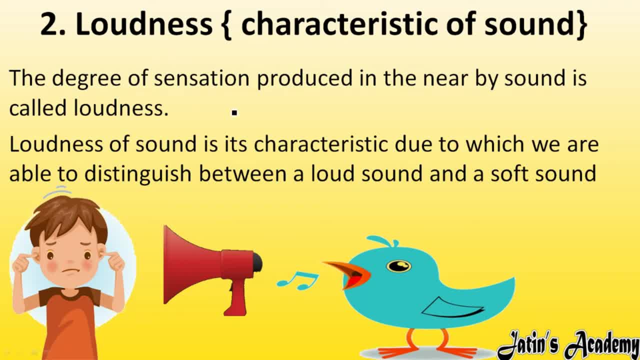 that is our musical scale. the musical notes of all the music are matching with that. now we are having second characteristic of sound, that is loudness of sound. so we have read: first characteristic of sound, that is pitch. now we are having second characteristic of sound, that is loudness. 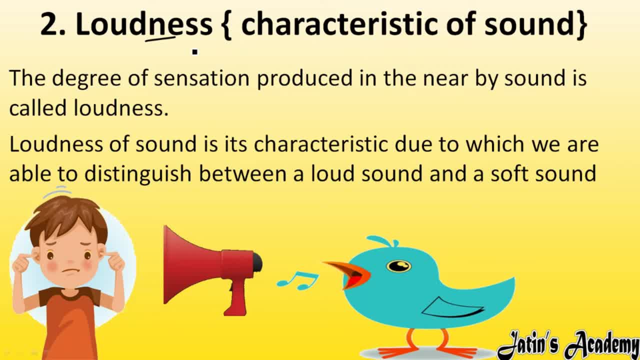 so what is the meaning of loudness, as the name suggests, loudness- how loud is a sound, or how faint is it? how high is it or how low is it? that is what we call loudness. the degree of sensation produced in nearby sound is how loud or how faint is the sound? 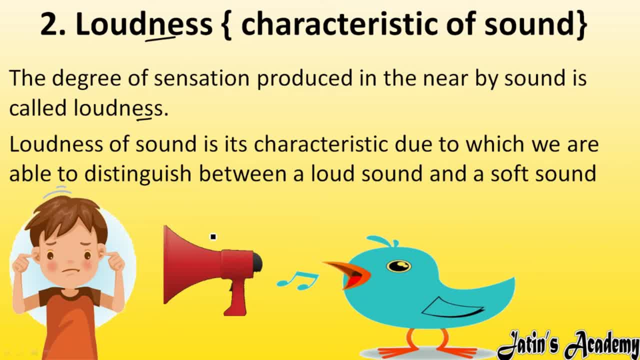 that is what we call loudness, like speaker. what is the loudness of speaker more or less? loudness of speaker is more. and here we are having bird. what is the loudness of bird? more or less? loudness of bird is always less so. what is the sensation of sound produced by the nearby object? 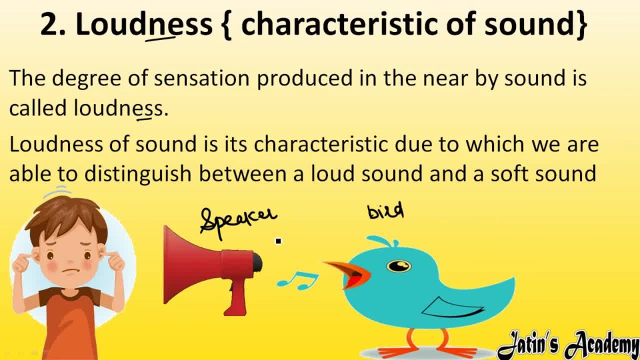 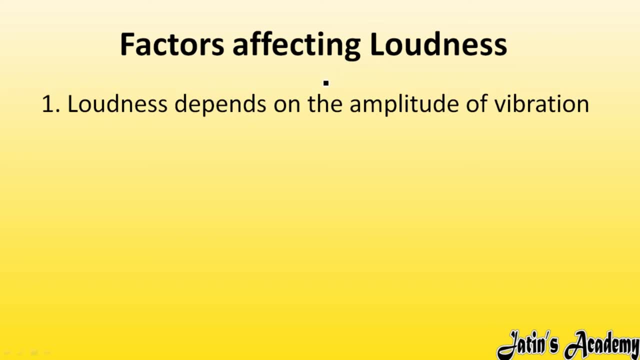 that is what we call loudness. so loudness is a characteristic of sound. we distinguish how loud is a sound and how faint is the sound we call faint as fable and faint as soft sound. so next we are having factor affecting loudness, as we have read in the case of pitch. 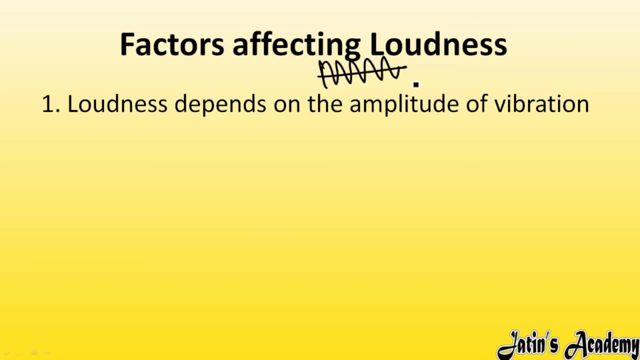 that the number of frequencies will be more. the number of frequencies will be more, the pitch will be more. and second, we are going to find out that the loudness depends on amplitude. if amplitude is more in one wave, then the loudness will be more. if amplitude is less in one wave, 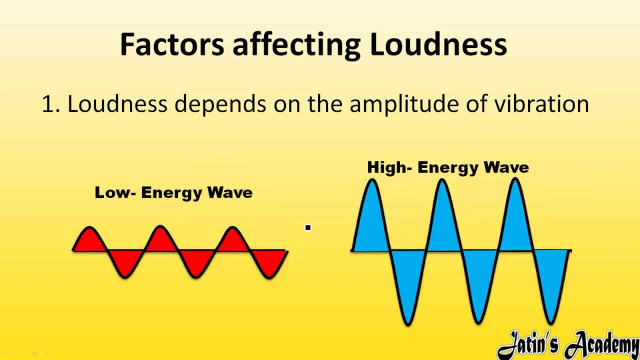 then the loudness will be less. here we are having the waveform for this, which is low energy wave, so the loudness of low energy wave will also be low. how is its wave low? see, if I am speaking very slowly means I am wasting my energy less. 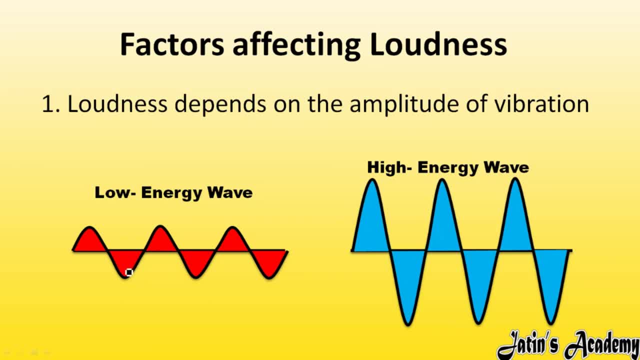 energy. less waste means that my sound will also be less. it has low energy wave and if I am speaking loudly, then what will happen? that I am using high energy. if it is high energy, then amplitude will be more, amplitude will be more and loudness will be more. 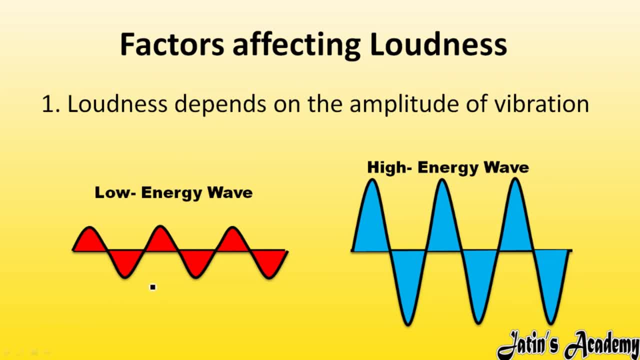 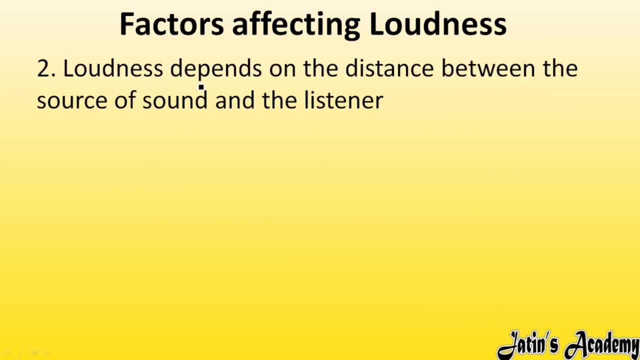 so more is amplitude, more is loudness, less is amplitude, less is loudness and amplitude is directly proportional. second factor affecting loudness is loudness depends upon the distance between the source of sound and the listener. if the source of sound and the distance between the source of sound and the listener 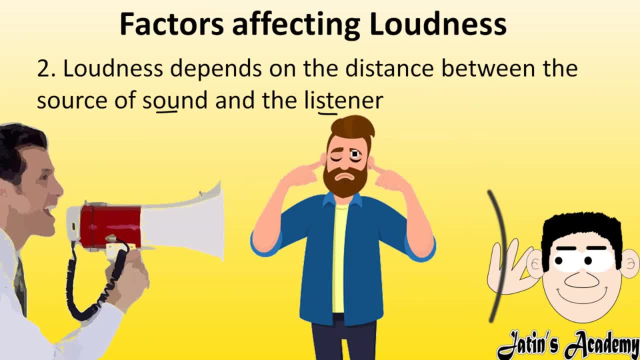 is very close, the source of sound and the listener are standing together, then what will happen? if the loudness is more and if the speaker is very far and I am standing far away, then what will happen? so it also depends upon the distance between the source of sound and the speaker. 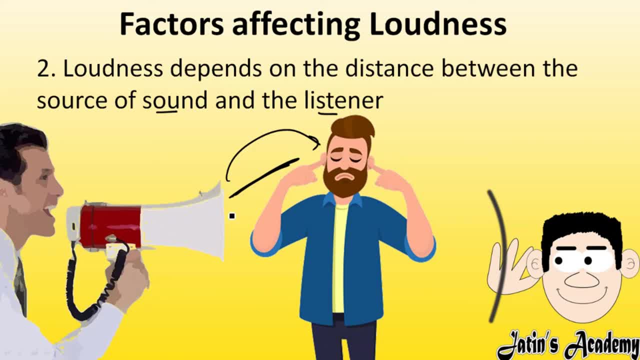 if there is less distance between the source of sound and speaker. if there is less distance between the source of sound and speaker, then more loudness will be there. and if more distance is there, then less loudness will be there. and if more distance is there, then less loudness will be there. 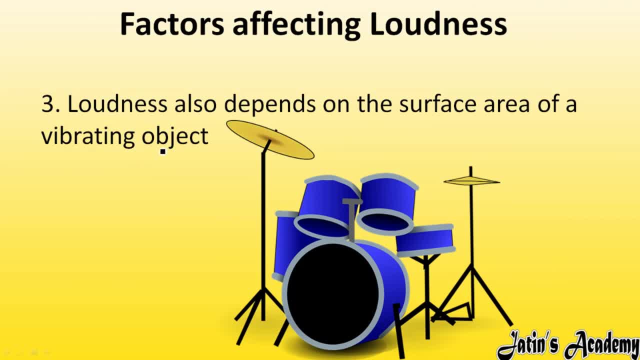 next factor of loudness we are having. loudness also depends upon the surface area of vibrating object. if surface area of vibrating object is more, like in this case, if surface area of vibrating object is more, then there will be more loudness. if surface area of vibrating object is less, 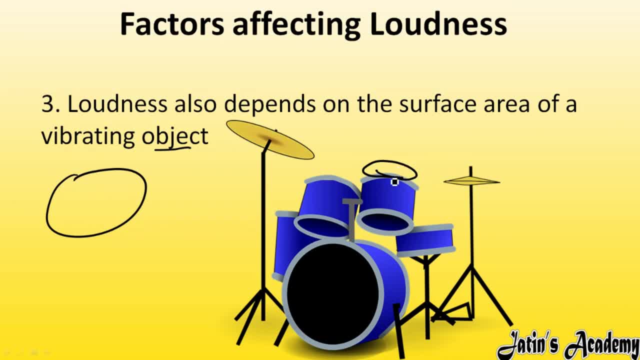 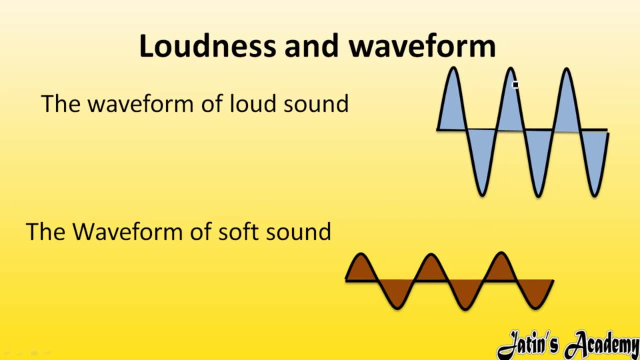 then there will be less loudness. if surface area of vibrating object is more, then there will be less loudness. here we are having the waveform and the loudness. if the amplitude waveform is more, then there will be more loudness. if amplitude in the waveform is less, 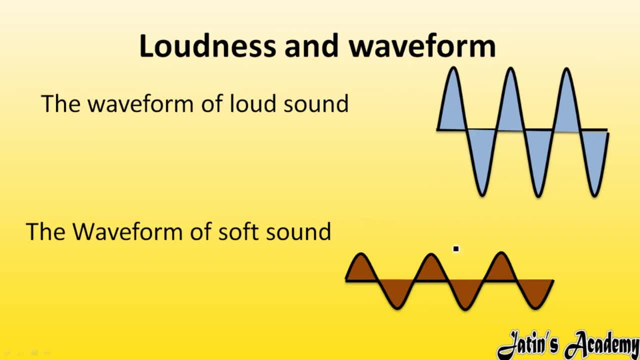 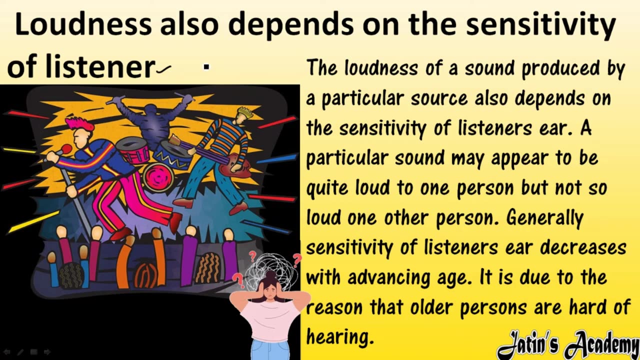 then there will be less loudness. so what can you do? you can see the waveform next we are having. loudness also depends upon the sensitivity of person. sensitivity of person means there are some people who easily listen to loud sound. they don't have any problem. but there are some aged people. 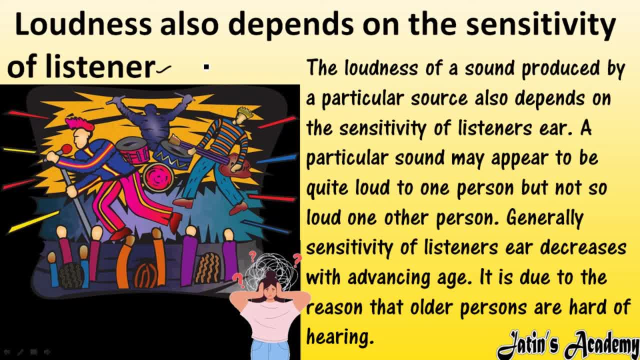 who don't like loud sound. they have headache, they don't like it. so it depends person to person. loudness of sound is produced by particular source of sound, but on producing particular source of sound, the person who is listening to the sound. it depends on his sensitivity. 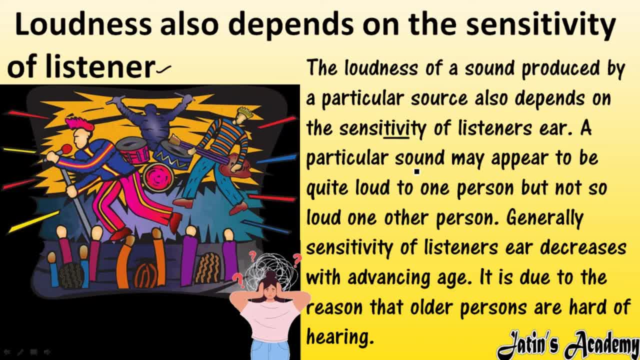 it depends on the sensitivity of the listener's ear, whether he is liking the sound or not, whether he is liking the music or the noise. like music is a decent sound. like music is a decent sound. like music is a decent sound. but the noise that makes our ears harsh. 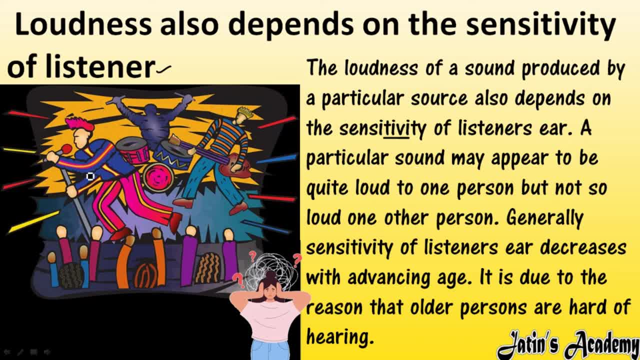 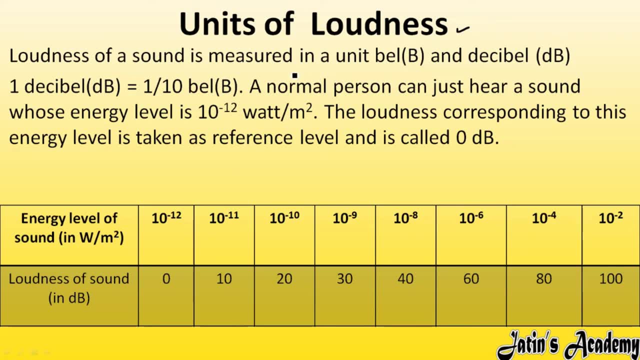 we call it noise. so for some people this sound will be good, but for some people this sound will not be good. it depends person to person. next we have units of loudness. next we have units of loudness. unit of loudness is measured in bell- actually, graham bell. 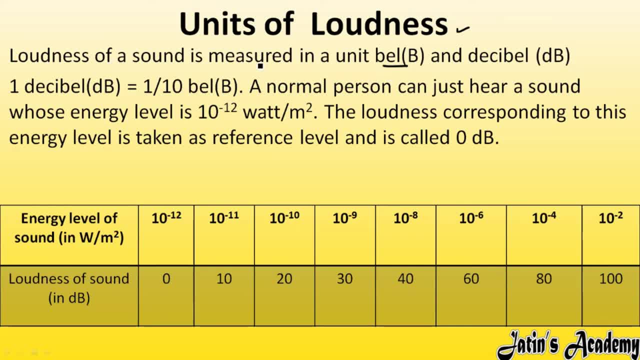 who discovered the telephone. we put unit of loudness that is bell and we represent it in decibel units. actually, the unit of loudness is bell, but in what values we use? we use loudness in decibel values. we use loudness in decibel values. 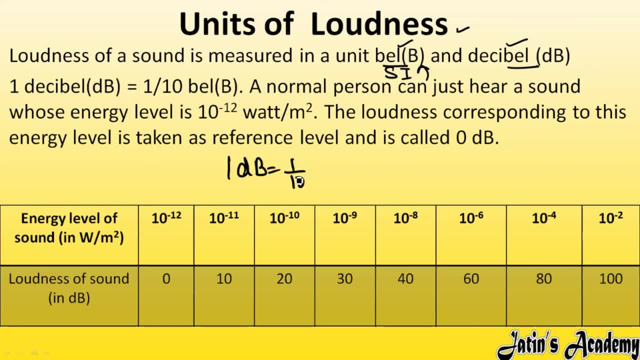 in decibel there is a 1 by 10 bell. deci means 1 by 10. deci means 1 by 10. a normal person can just hear a sound whose energy level is 10-12 watt per meter square. a normal person can. 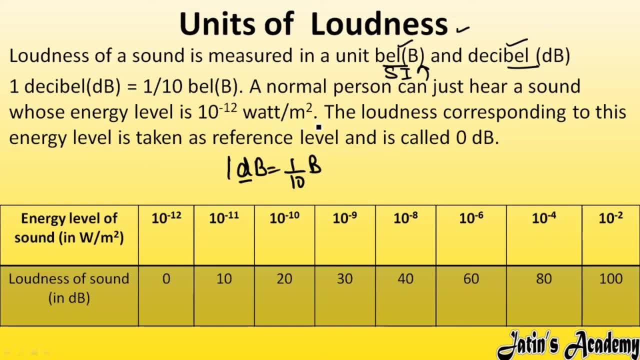 can hear the sound of 10 to the power of minus 12 watt per meter square and the energy of 10 to the power of minus 12 watt per meter square is called 0 decibel and the energy of minus 11 is called 10 decibel, 20 decibel, 30 decibel. like this we are having. 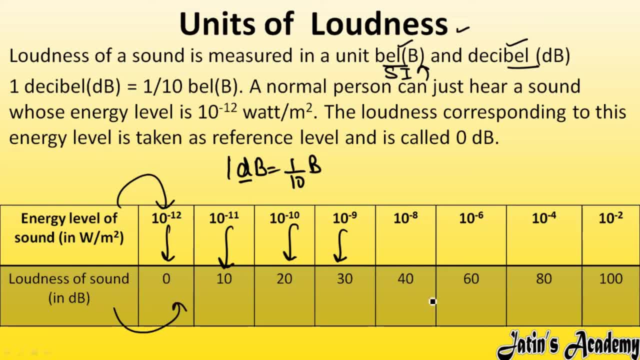 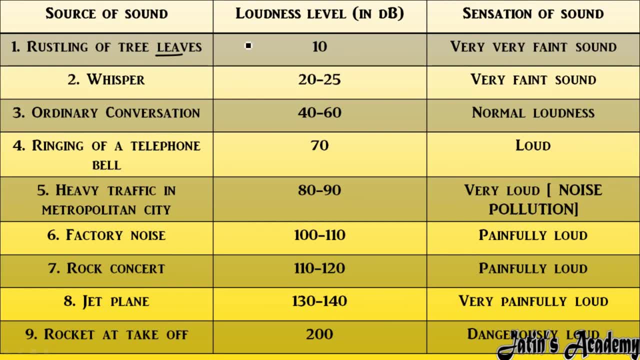 this is the energy level of loudness and this is the decibel values of loudness. so this is a chart. given that the rustling of tree leaves which move like this with the help of wind, the sound produced in it is 10 decibel sound, which is very faint, very, very faint sound. 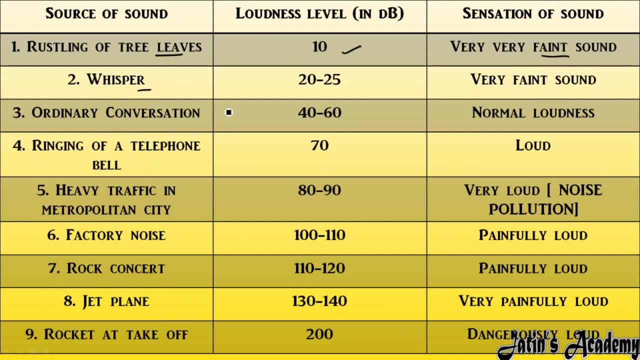 which we don't hear very well when we are whispering that something is spoken in the ear. something is spoken in his ear. the sound spoken in the ear is of 20 to 25 level sound of 20 to 25 decibel. 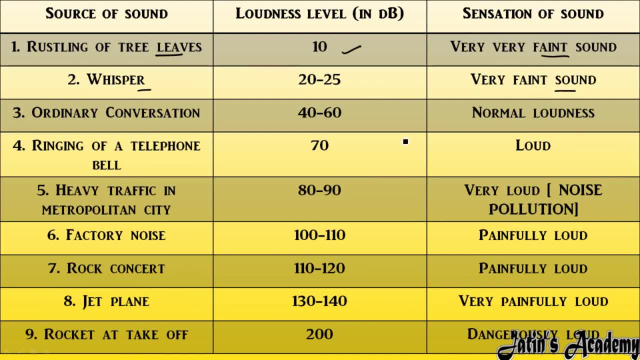 which is very faint sound, which is very difficult to hear. when we are having an arm conversation, then the sound is 40 to 60 decibel. that is normal loudness which we can hear normally. then we are having ringing of telephone, then we are having ringing of bell. its loudness is 70 decibel. 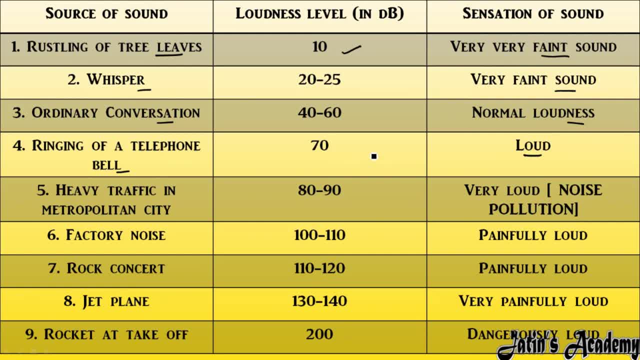 which is a loud sound, means its loudness is a little more than the normal loudness. next, we are having heavy traffic in metropolitian city. when there is heavy traffic, the sound of horn on horn is 80 to 90 decibel, which is a very loud sound. 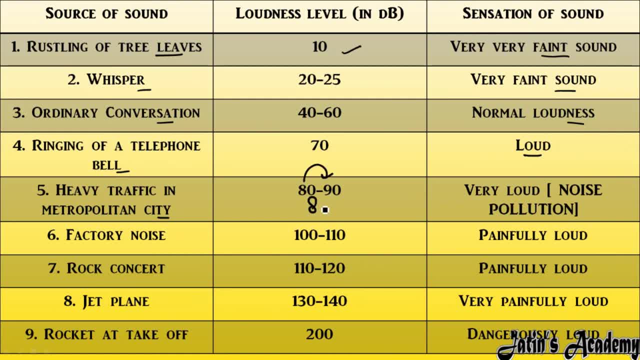 and the sound above 80 decibel is called noise pollution, which is very harmful for our ears, for our mind also. so what will happen? the sound above 80 decibel is called noise pollution. then we are having factory noise. how much noise comes from the factory? 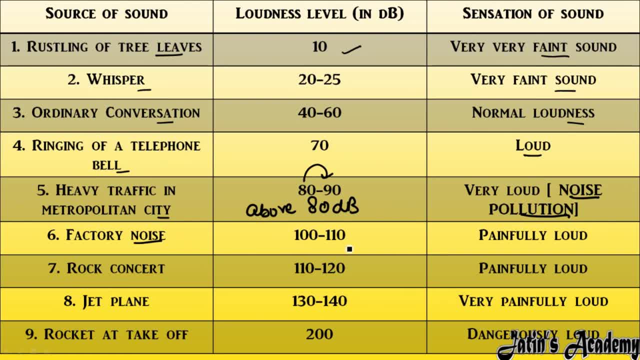 its loudness is 100 to 110 decibel, which is painful loudness, means our ears start to hurt. so next we are having rock concert. rock concert is music. DJ is playing in that 110 to 120 decibel, which is very painful loudness. 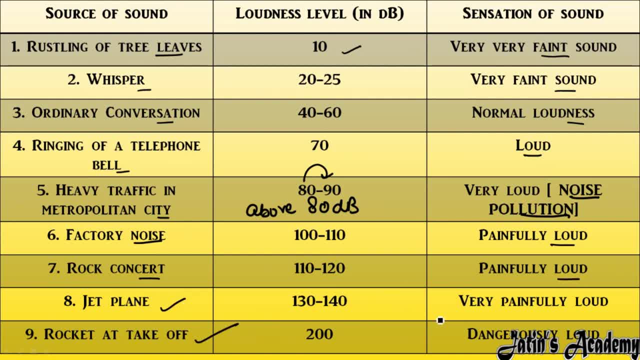 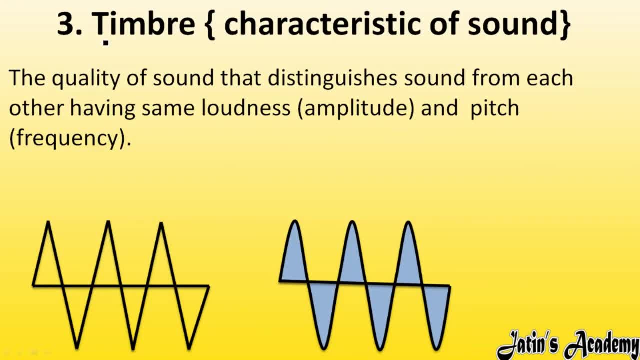 next we are having for jet plane rocket at take off. all these are very painful and rocket at take off is very dangerous and it can damage our ears. so next we are having third characteristic of sound, that is, timber. so what do you mean by timber? 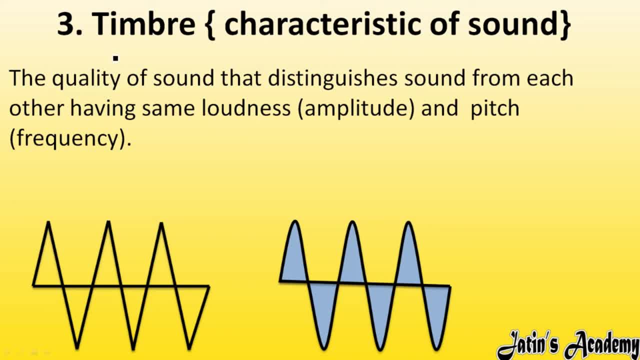 see carefully, actually in timber, it is the quality of sound means we always distinguish the quality of sound. for example, here we have two ladies standing in front of me. one of them is my mother and one of them is my teacher. for example, my eyes are closed. 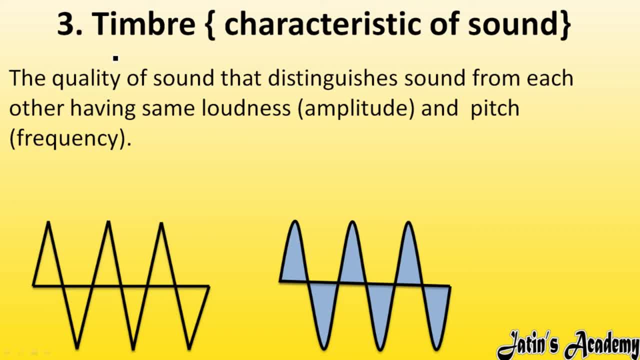 and two ladies are standing in front of me. one is my mother and second is my teacher. ok, so if I close my eyes and my mother is speaking, so I will understand after closing my eyes that she is my mother, or if my teacher is speaking. 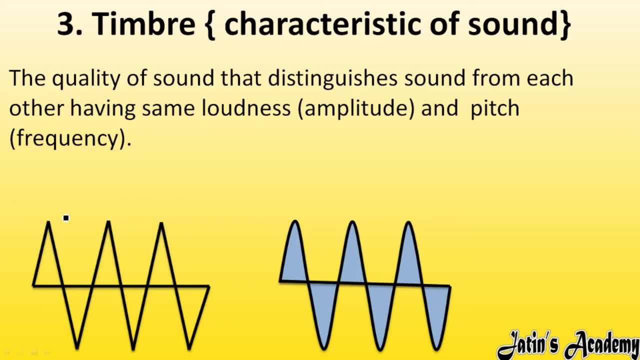 I will understand after closing my eyes that she is my teacher. how will you understand, for example, my mother and my teacher? their loudness is same, their loudness and their amplitude and their frequency for the same second and same time, same number of oscillations. 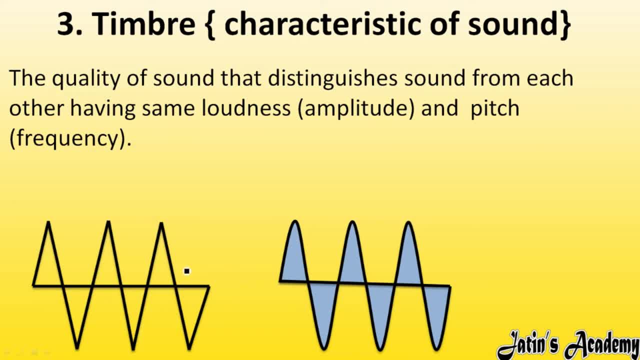 same number of time and same oscillations if their loudness and amplitude and their frequency is same, both loudness and amplitude, and frequency and pitch is same, but still I can distinguish who is my mother and who is my teacher by the characteristic of sound known as timber. 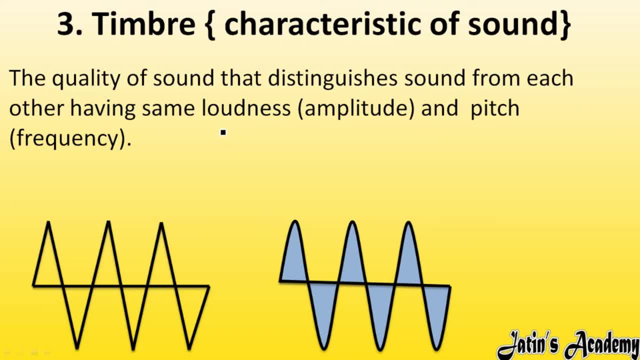 so timber distinguishes sound from one sound to another. sound, actually how sound is differentiated in both sound. frequency and amplitude is same, loudness and pitch is same, but waveform is different. waveform is something like this and waveform is something like this. so, with the help of waveform, 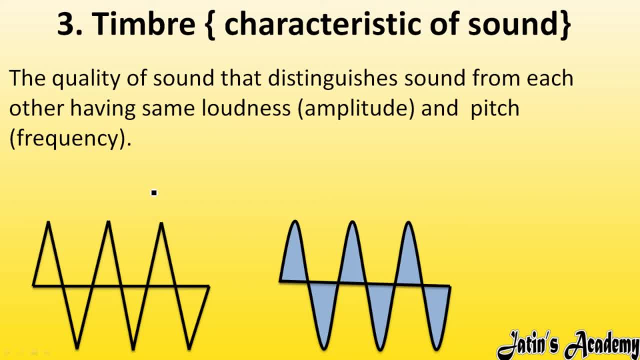 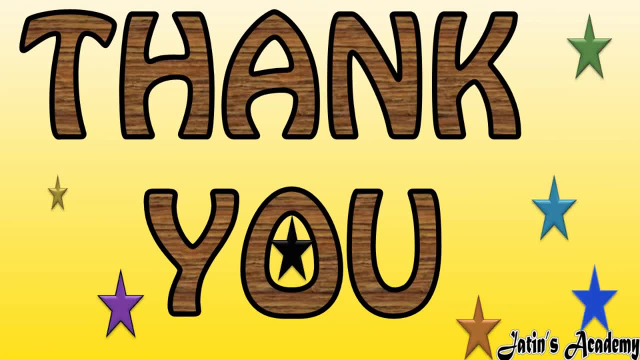 I can distinguish between my mother's voice and between my teacher's voice, and this is known as timber. so this is all about our chapter number 7. that is sound of class 8 ICLC physics. if you like the explanation, please like it, share it and subscribe our youtube channel. thank you so much.